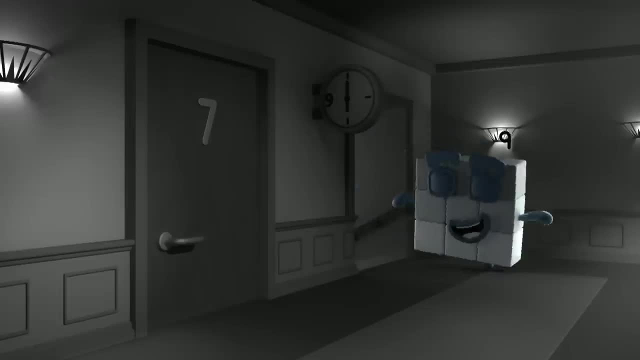 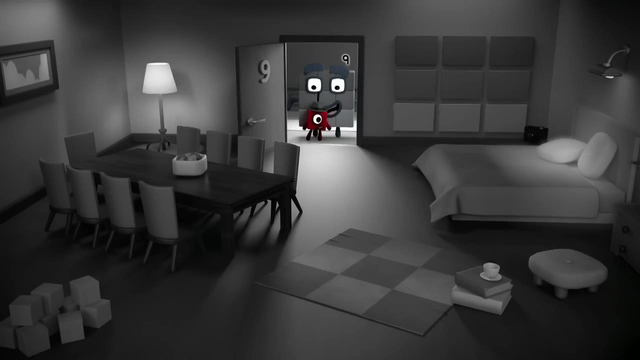 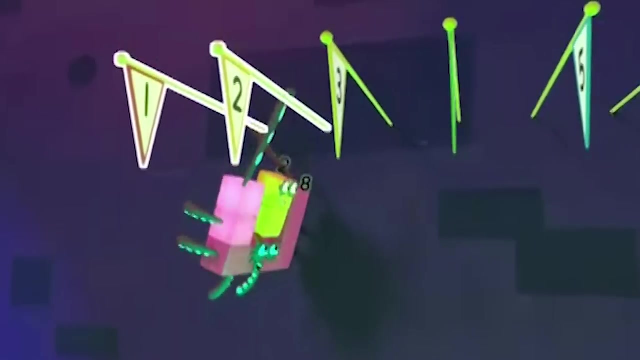 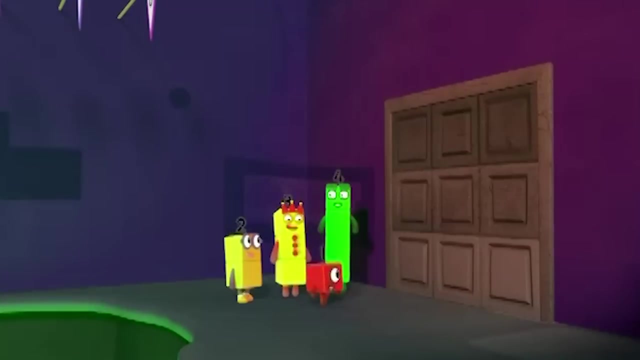 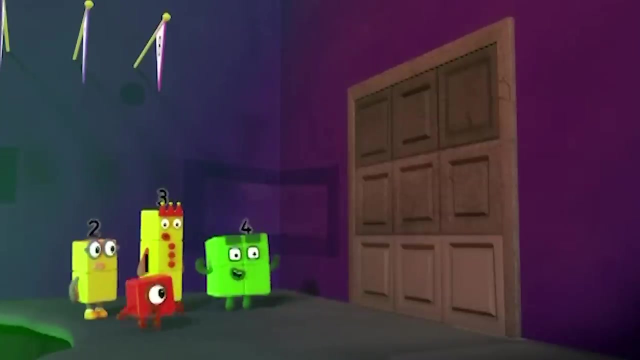 So my things must be Right where I left them. Case closed. You can count on us with an OtterBox One, two, three, four, five, six, seven, eight Swing. Oh, It's stuck. Squares are strong. 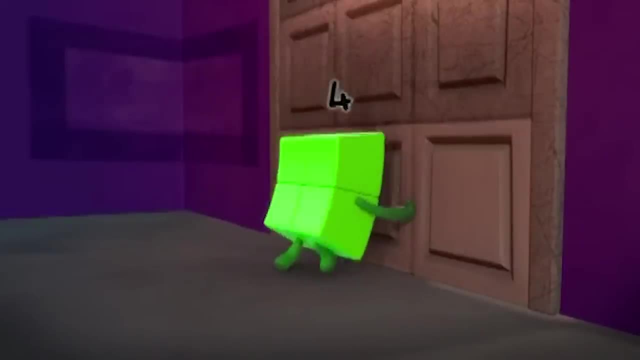 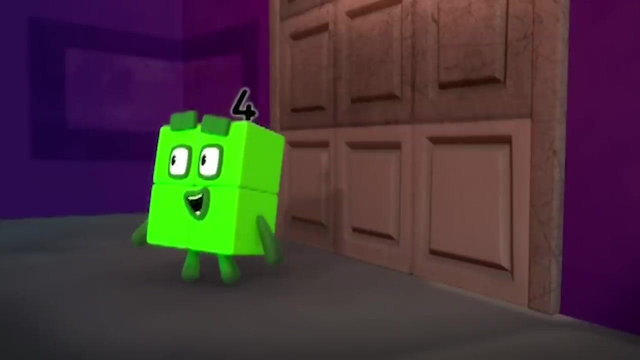 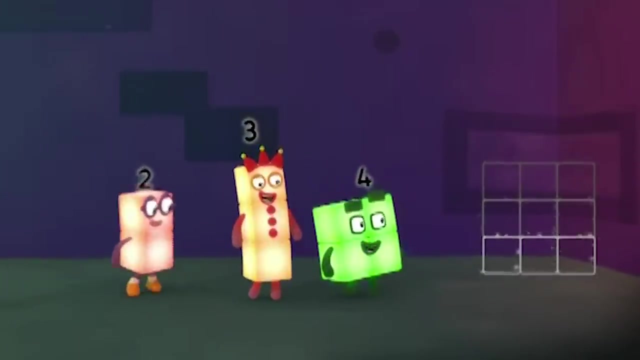 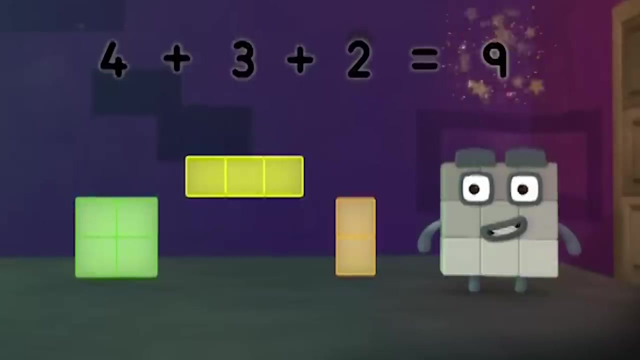 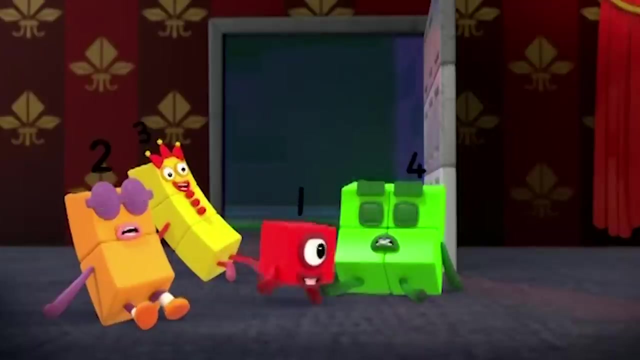 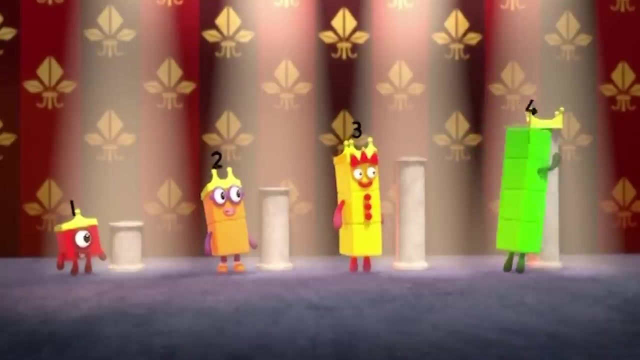 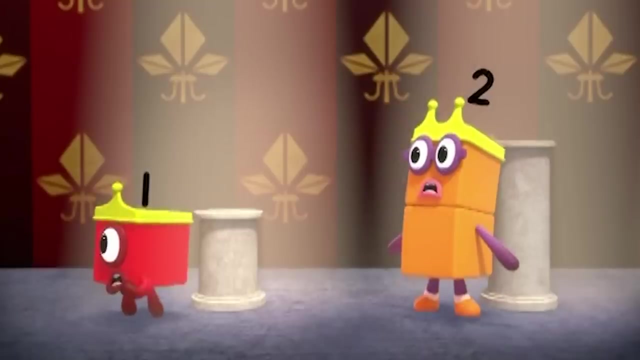 Let me try. We need a bigger square. Nine: How do we get nine? Three, Four Plus three Plus two Equals nine. Thanks, One, Two, Three, Four, Four crowns, Cool, Uh-oh. 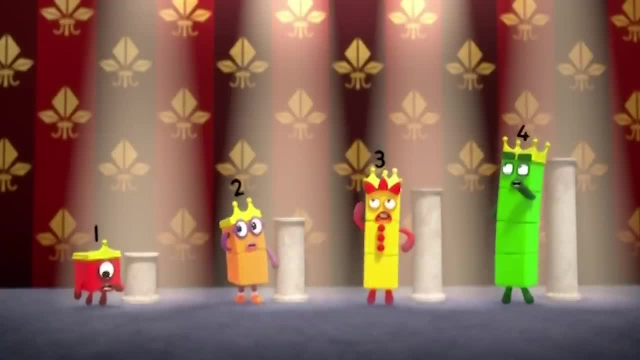 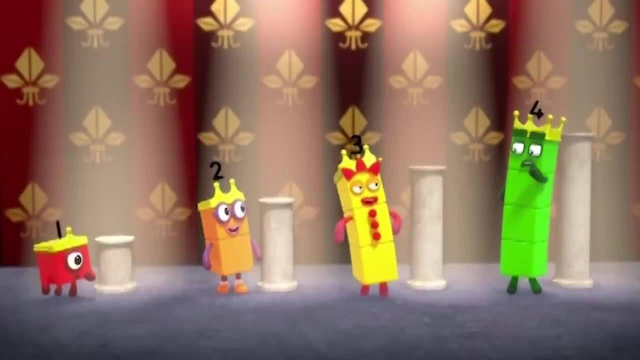 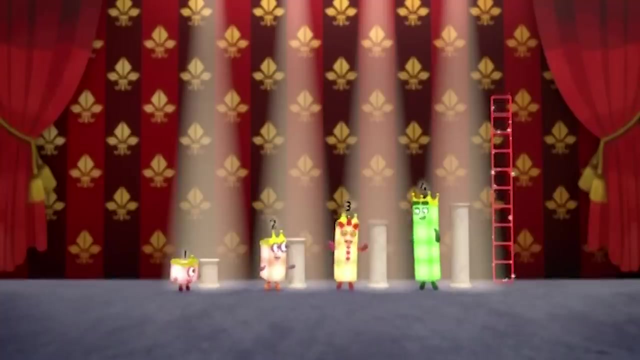 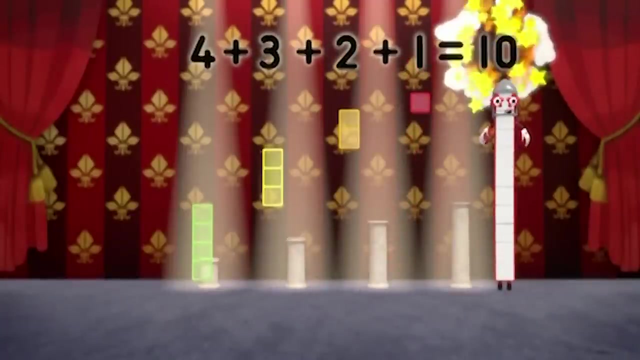 How are we gonna get out? Ah Ooh, If ten was here, we could rocket out through there. How do we make ten All together? now, Four Plus three Plus two Plus one Equals Ten, Ten. 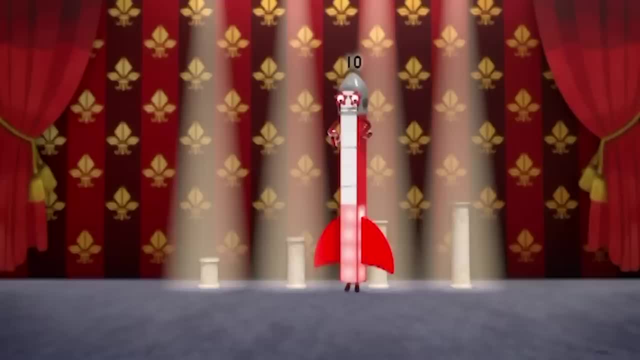 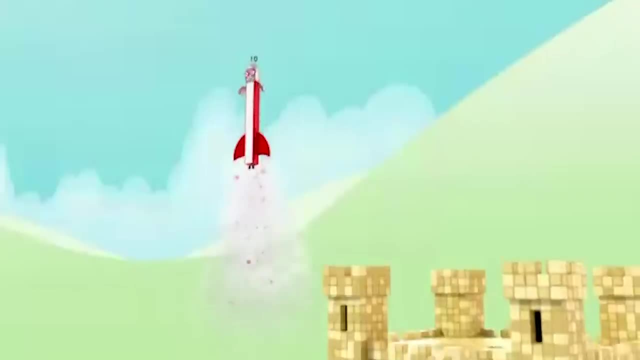 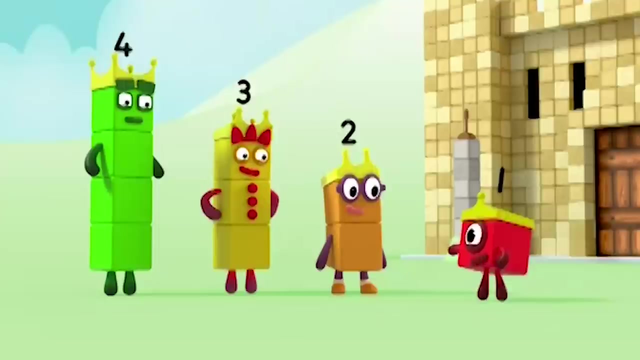 Nine, Eight, Seven, Six, Three, Two, One Blast off. Four, Three, Two, One. What an adventure. We may be little numbers, but when we work together we're still the kings and queens of the castle. 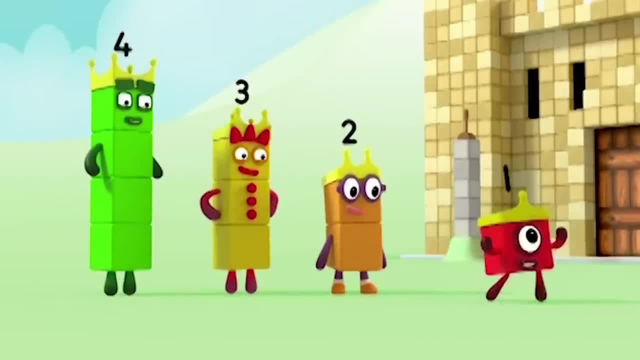 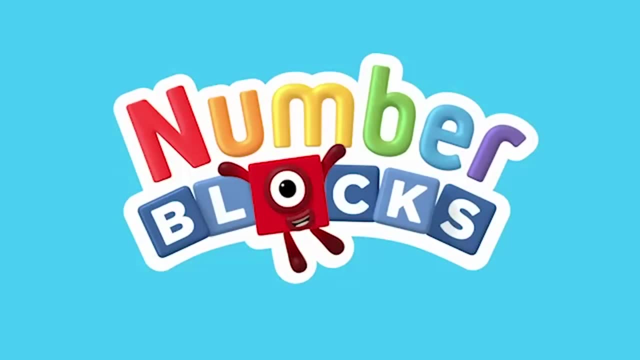 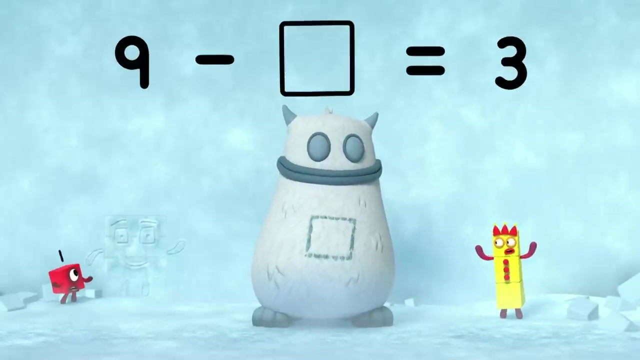 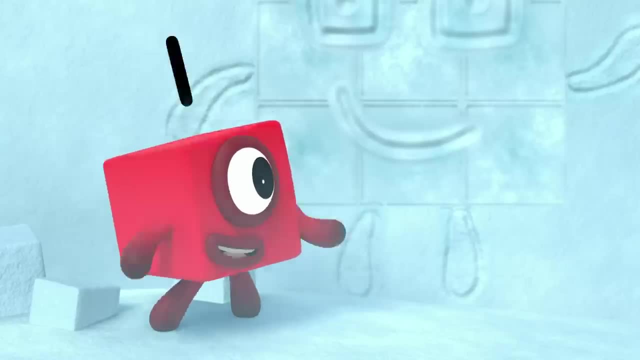 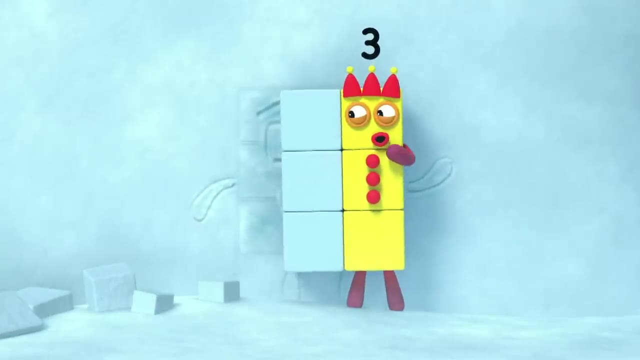 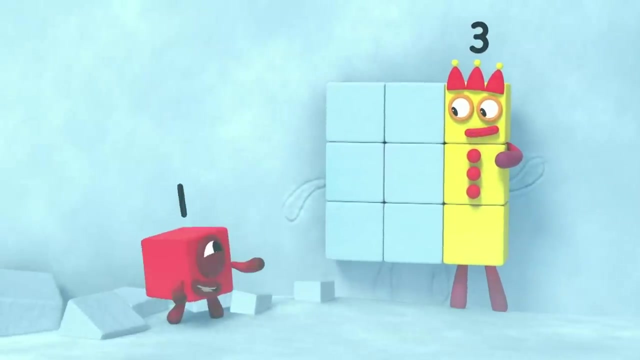 Number one: Young, Young Equals 3.. So what's missing? Hmm, Come over here, Three, Hi Brrr. That's one, Two, Three, Four, Five, Six There. So that's what's missing. 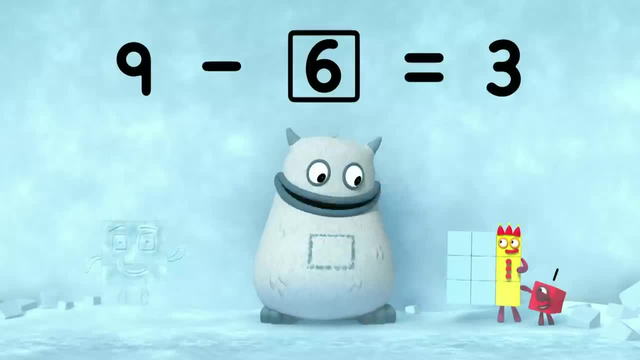 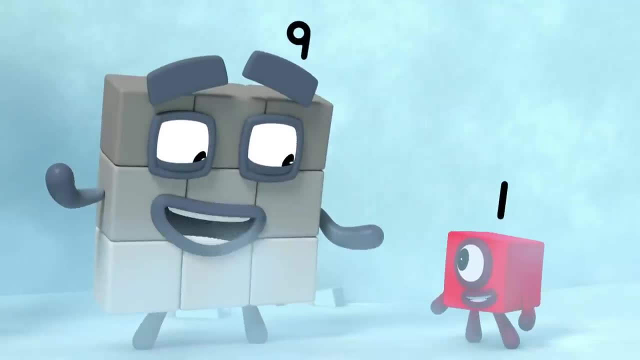 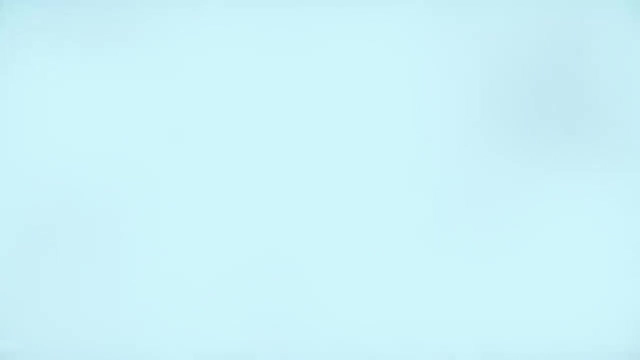 Nine minus six equals three Yum-yum. well done, Hooray. It's good to be back. Where are the others? Octoblock's legs? Yum-yum, yum-yum. Everybody stay close. No need to panic. 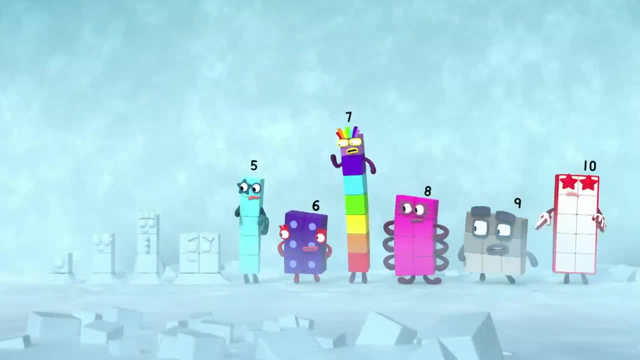 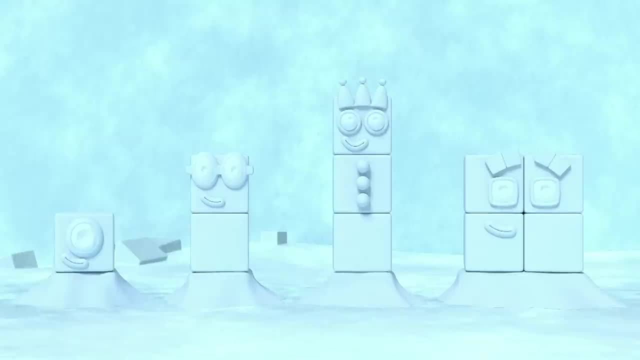 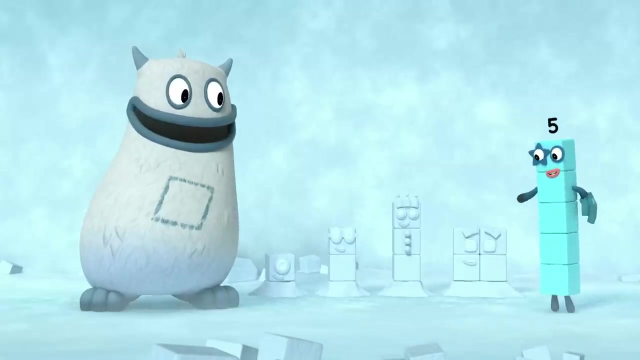 Um, What's wrong, friends? Why don't you? Oh, they're made of snow, Snow, Yum-yum. who's in my tummy? Who's in my tum? That's easy. The real one, two, three and four. 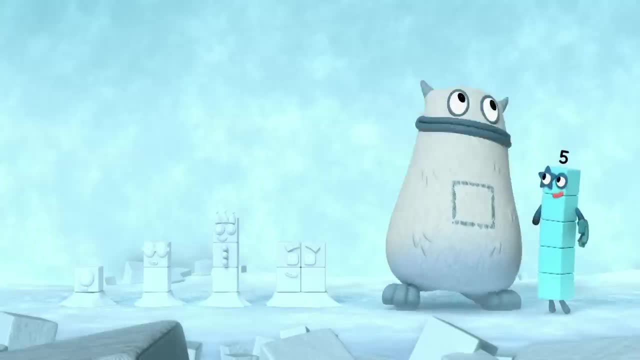 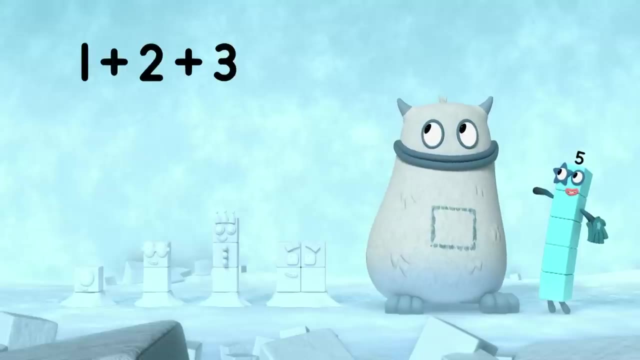 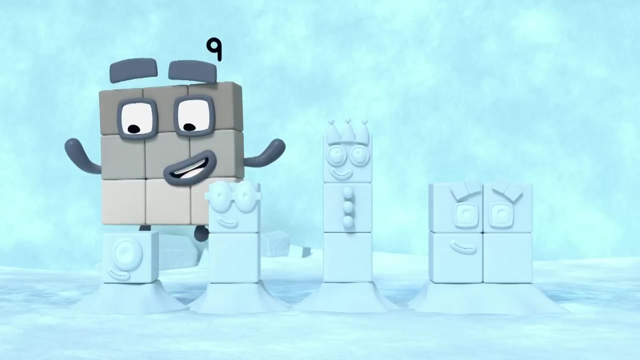 No, they're all together now. So what do they make when they're all together? One plus two plus three plus four equals Yum. Let's try adding the snow blocks together: One, two, three, four. One two, three, four. 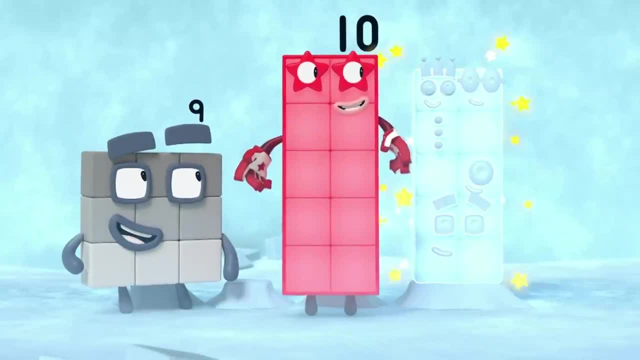 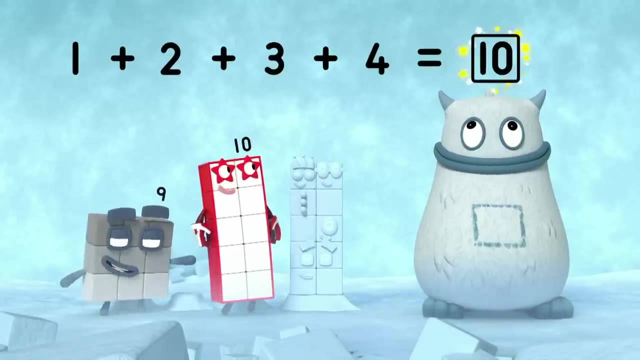 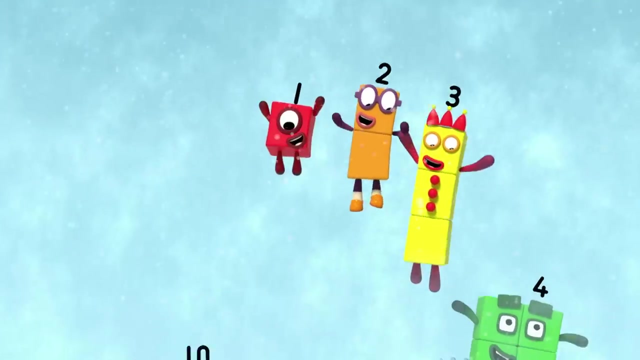 five, six, seven, eight, nine, ten, Ten snow blocks. So one plus two plus three plus four equals ten. There's a ten in your tum, Yum-yum. well done, Hooray, It's nippy out Much warmer inside. 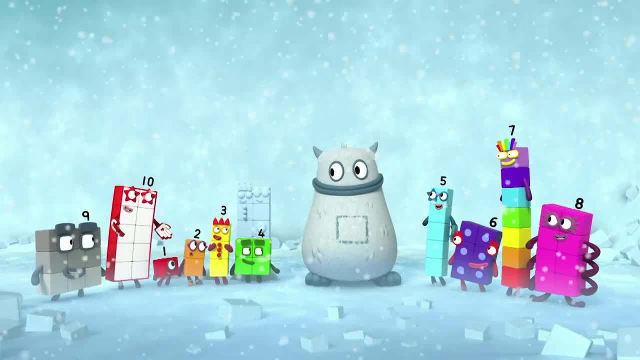 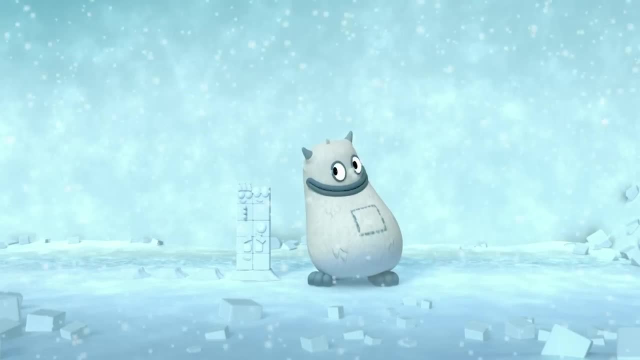 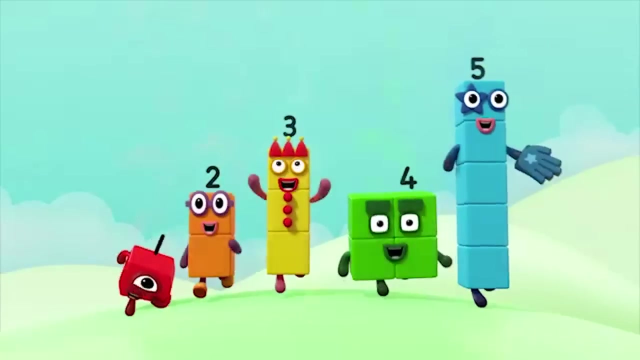 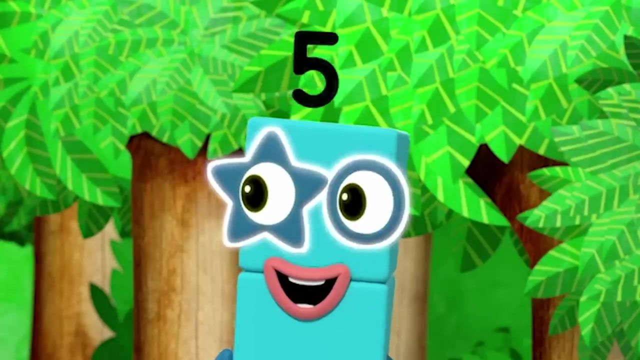 Can we all come in until it stops snowing, please? No problem, Hooray, Hooray, And plenty of room for you too. You can count on us with another box. How many eyes has it got? One, two, three arms. 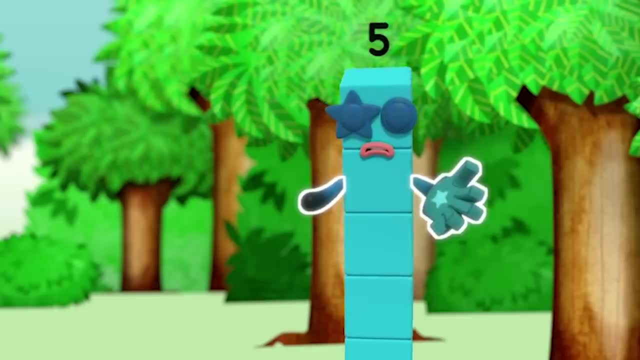 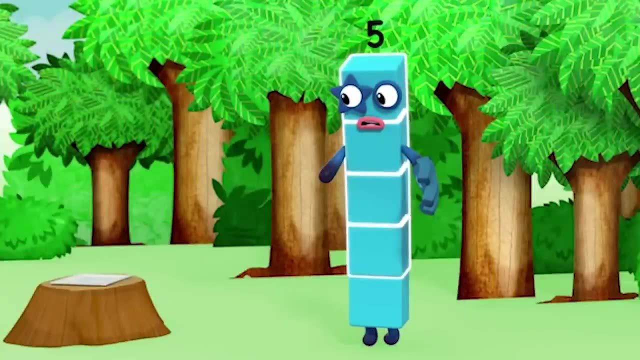 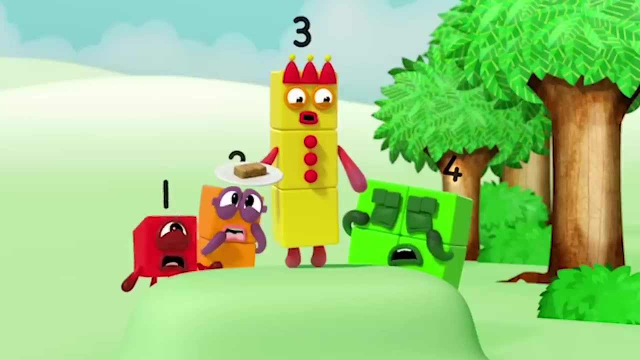 How many arms? One, two, three arms? How many blocks? One, two, three, four, five, Three blocks. It's the Flapjack Snapper. No, it's five. What are you all doing? Five. 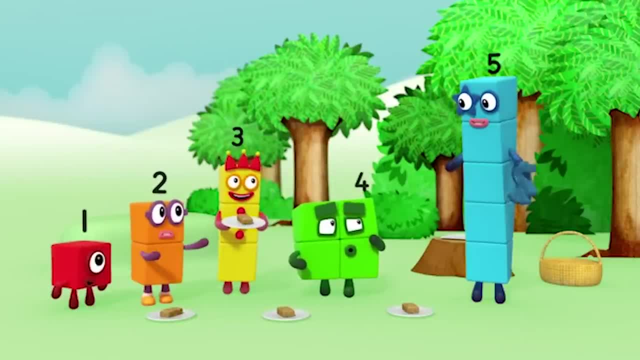 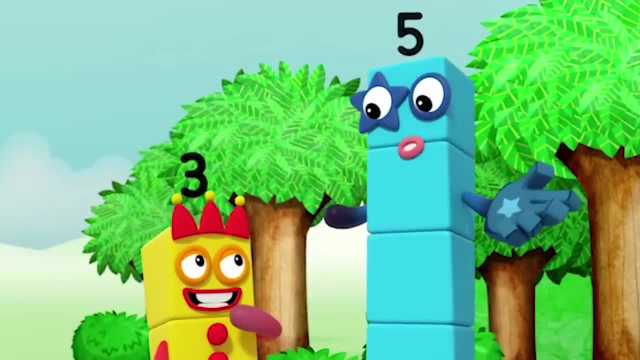 You haven't got three eyes or three arms. Whoever told you I did? Hmm, I counted them Three. Do you know how to count? Yes, of course. Look at a bunch of things, Say some numbers and then say three. 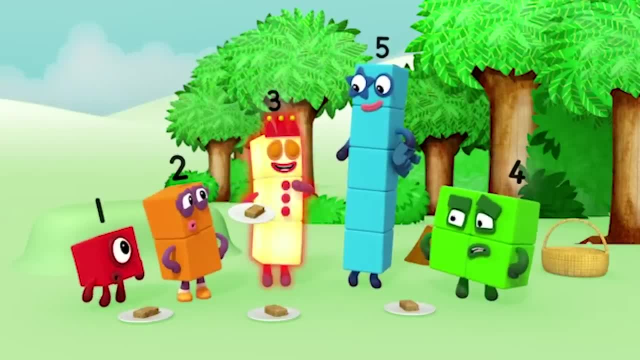 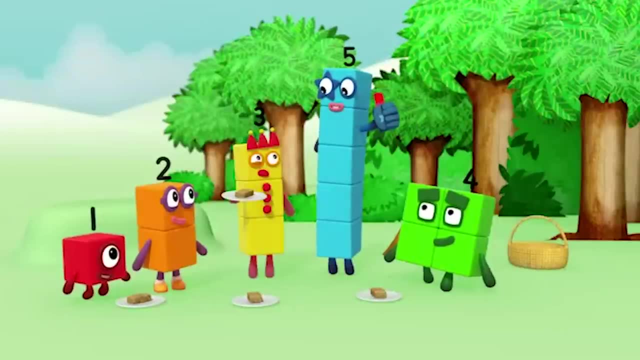 Because three's the best number. There's a little more to it than that Three. There are some rules you have to follow. Rule one: Count everything once. Try counting those flapjacks. It can help to put them in a line. 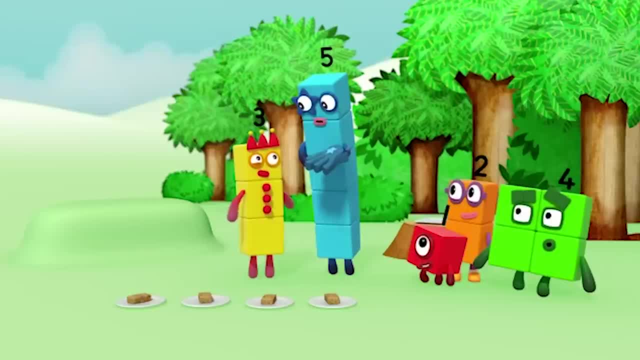 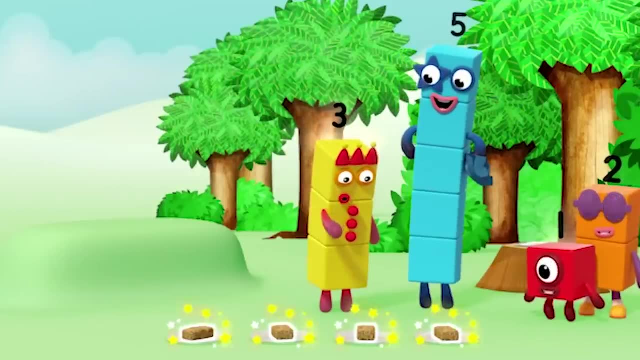 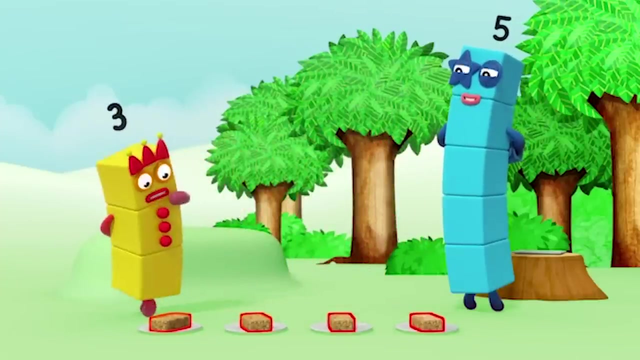 and to point at them one at a time, to make sure you don't miss any Or count the same one twice. One, two, three, Four. Very good, Four. three, two, one, Wait one. That's not right. 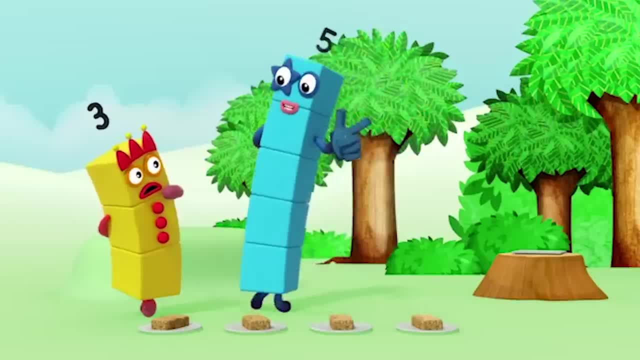 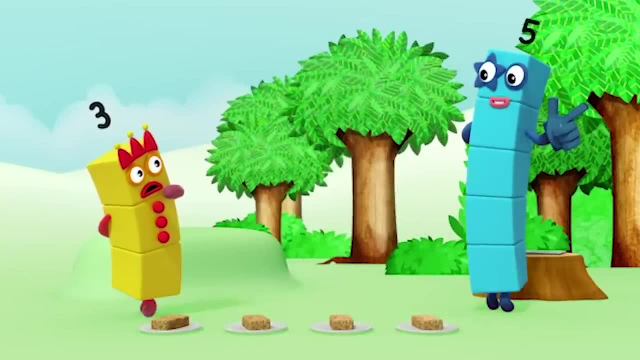 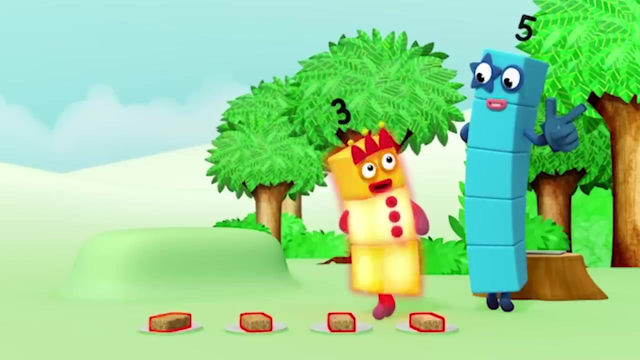 Rule two: Say the numbers in the right order. If you don't say them in the right order- one, two, three, four- you won't know how many there are. Oh, One, two, three, four, Three flapjacks. 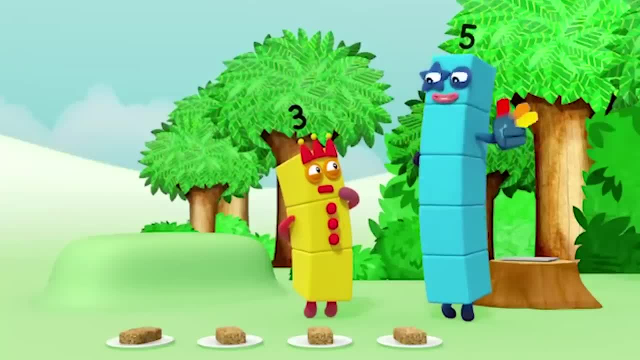 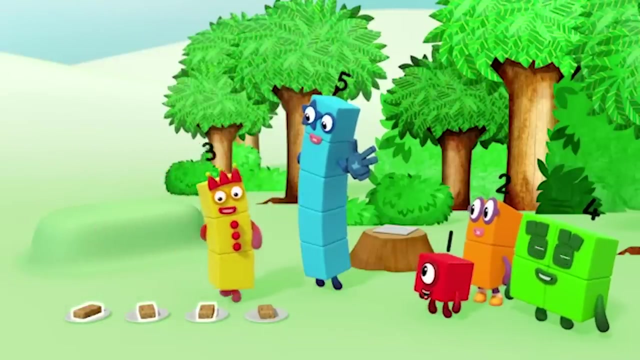 Oh, we've been here before. Rule three: The last number is how many? When you reach the last thing to count, the last number you say tells you how many there are. Try, You can do it. Go on One, two, three, four. 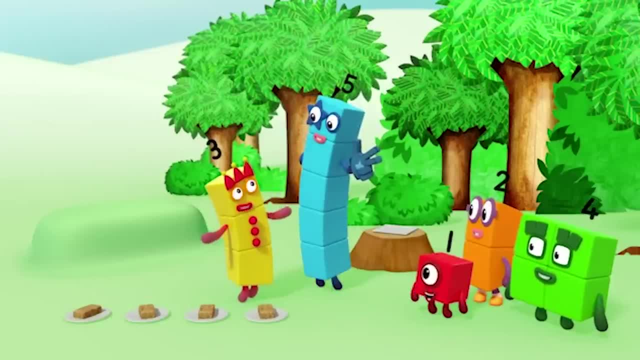 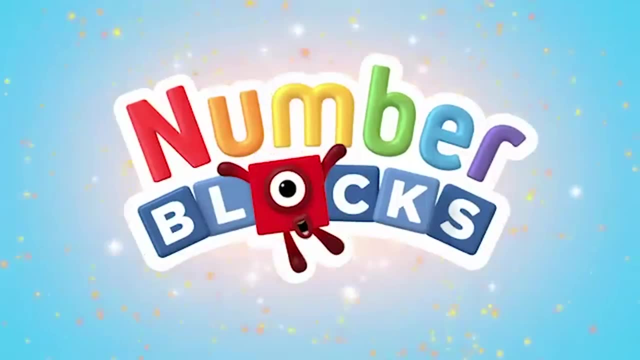 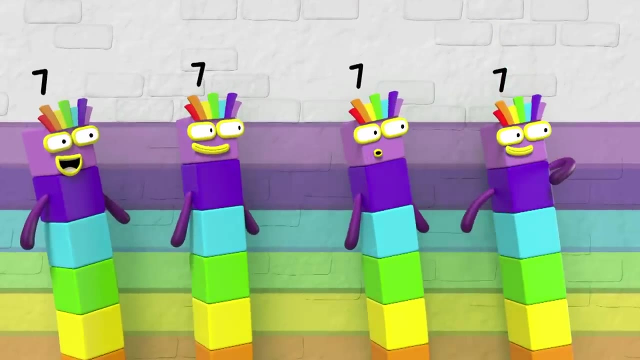 That's the last flapjack. So four flapjacks, That's right. Yeah, You can count on us with another box. I'd love to be you, but I come up short. I need to add something, but what? 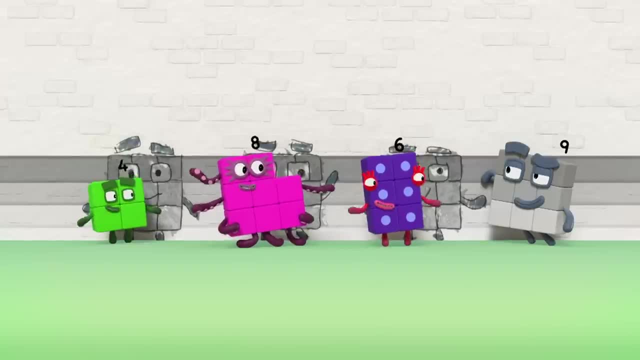 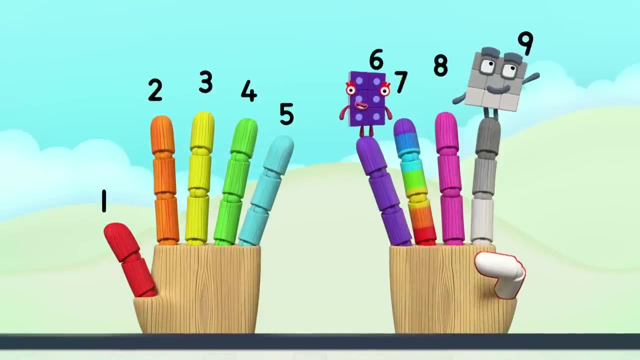 I'd love to be stronger, like: nine is What have you got? if we haven't got, You can count on your hands. Seven, eight, nine, That's the difference. Three, One, two, three. You can fill in the space. 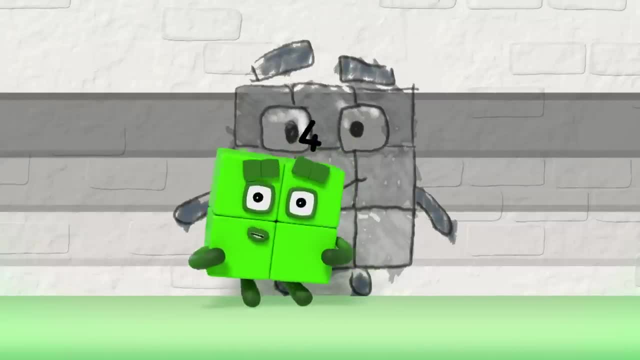 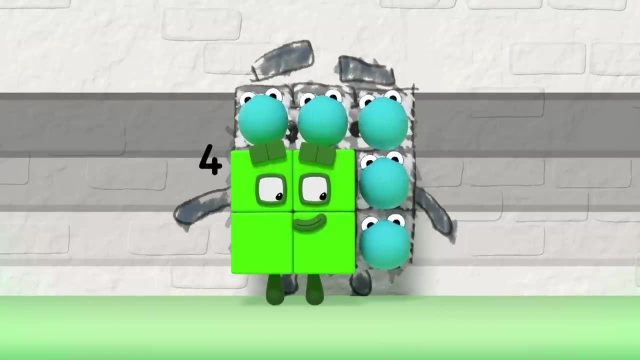 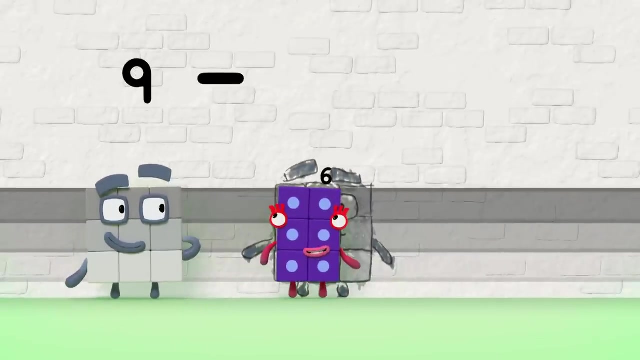 That's the difference. One, And if the difference won't pop into your head, you can count number gloves in place: One, two, three, four, five, Five. The difference is five. So what's the difference? Nine minus six equals three. 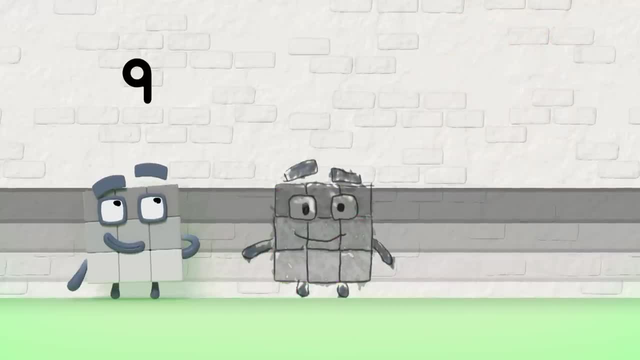 That's the difference. Three Nine minus me equals one Three. That's the difference. One Nine minus four equals five. That's the difference Five. So make up the difference and everyone will see what the difference is between you and me. 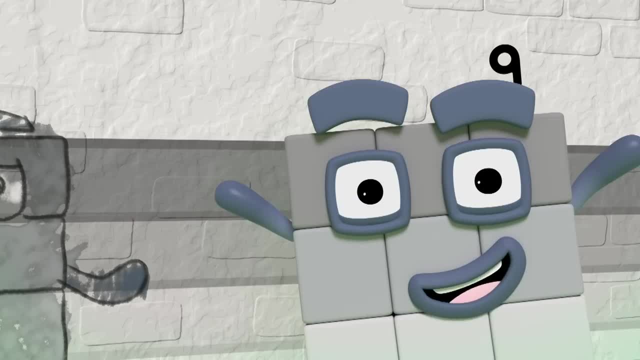 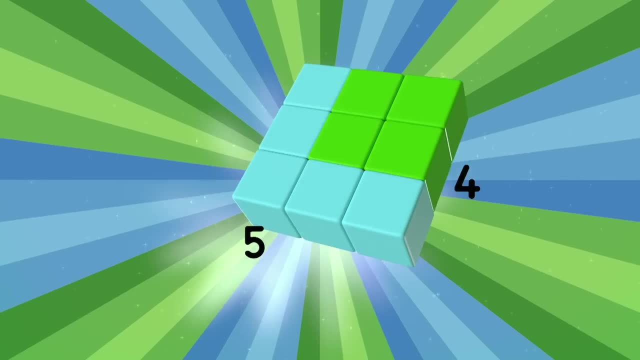 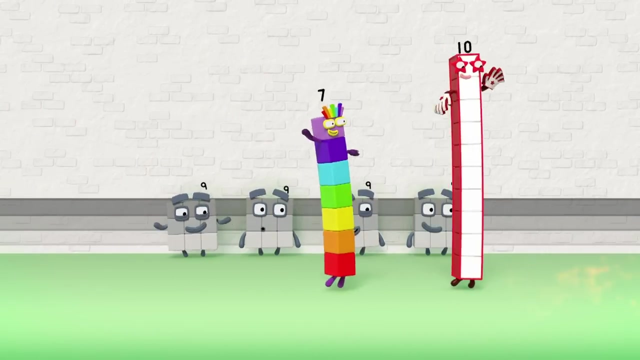 I'd love to be you, but I'm much too big. One Two, Three. One Two, One Two, Three, Two, One Two, Two, One Two, Two, One, Two, Two, Two. 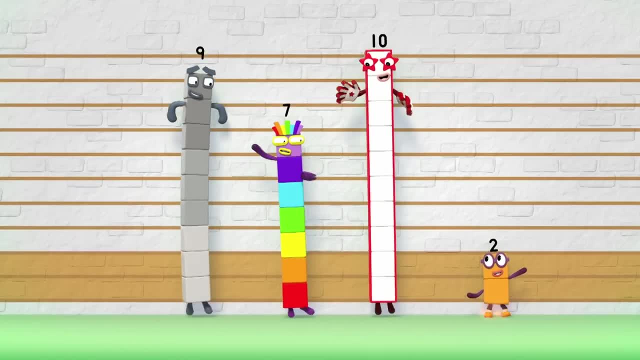 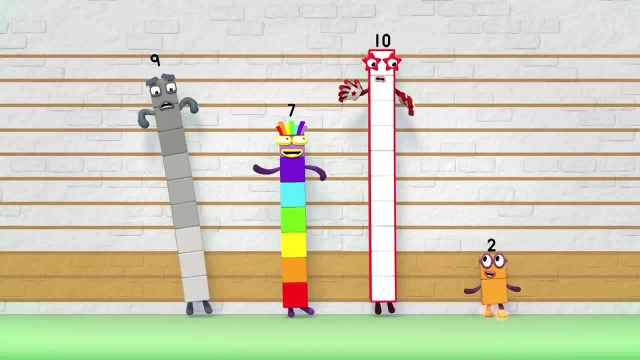 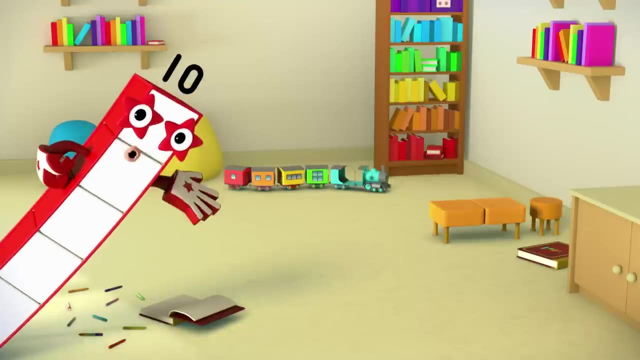 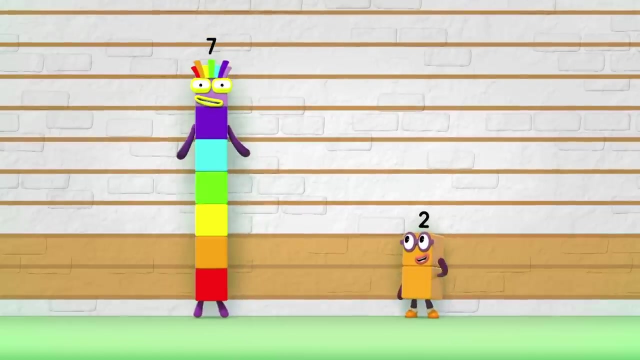 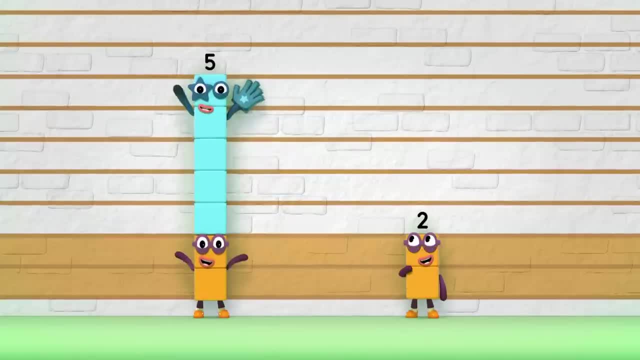 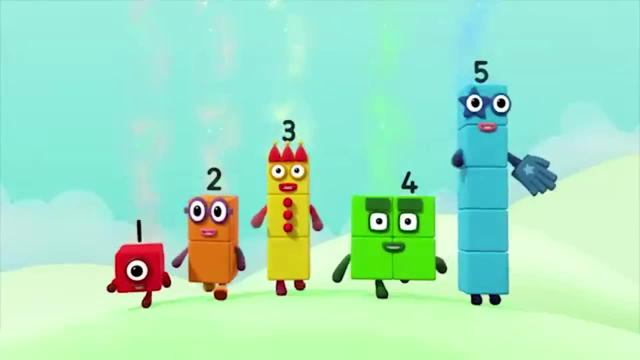 One, Two, One, Two. What's the difference? Five, So What's the difference? You can count on us with another box. Box equals two plus two. Yum, yum, Yum, yum, No, no, no, you silly machines. 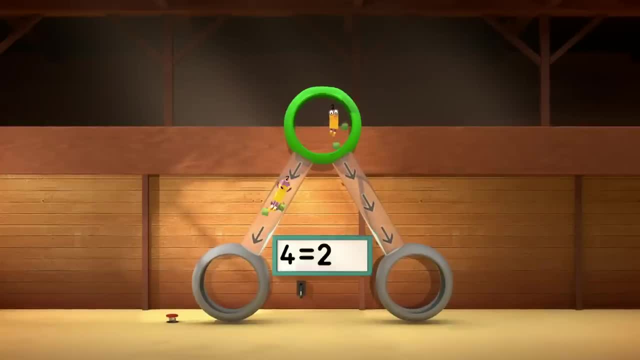 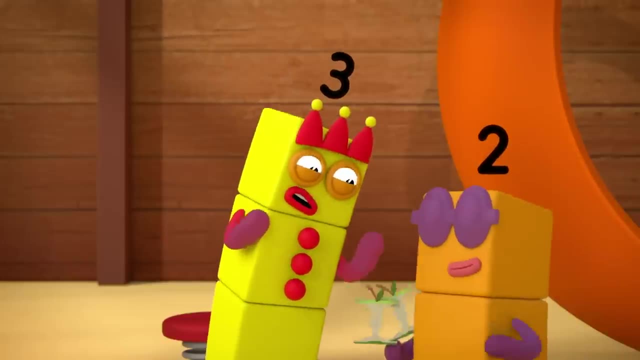 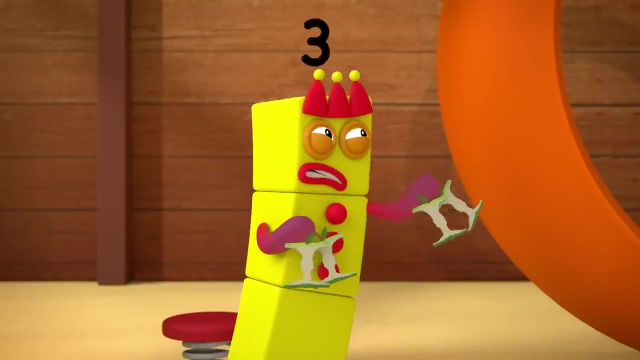 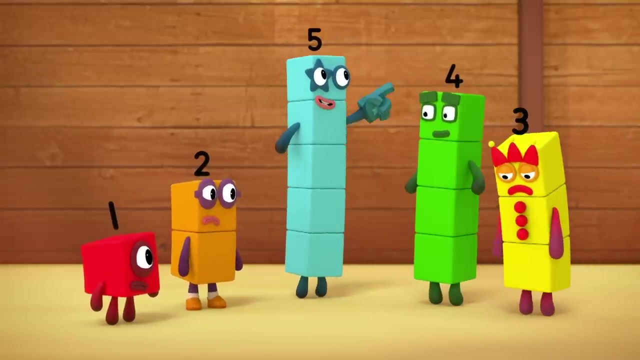 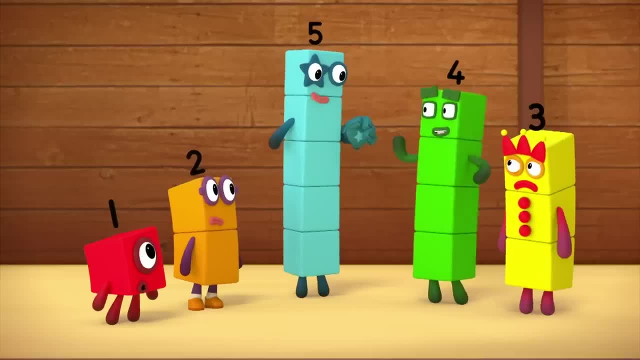 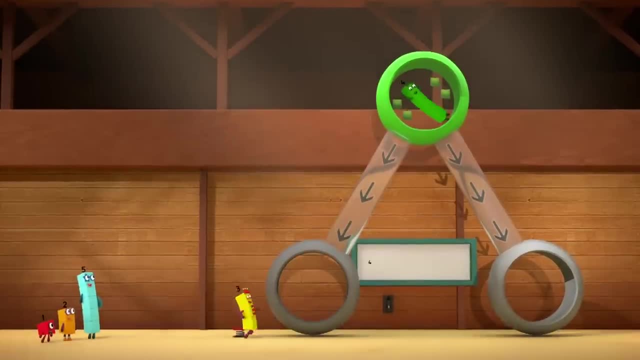 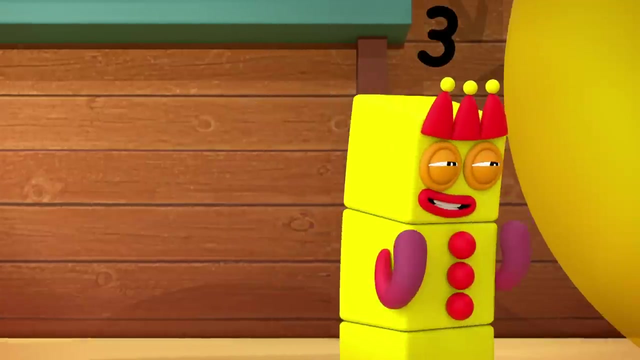 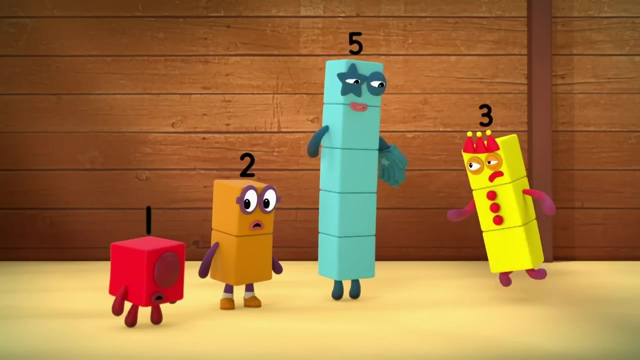 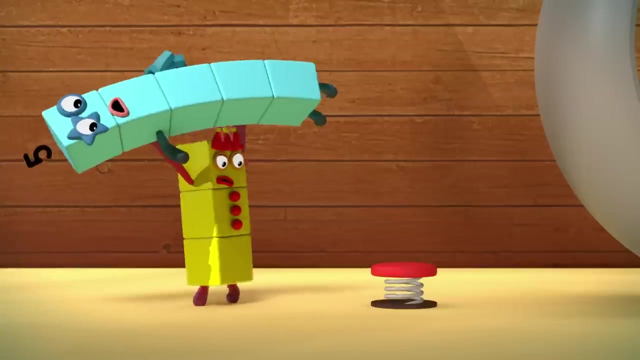 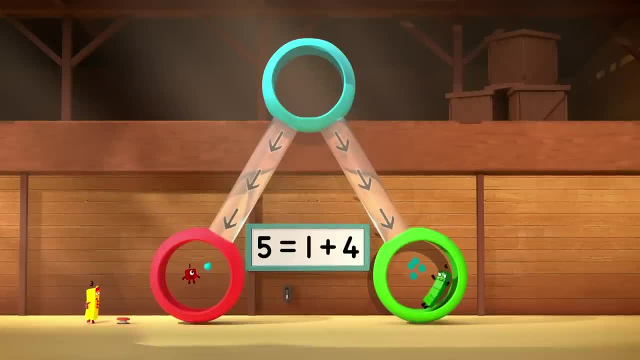 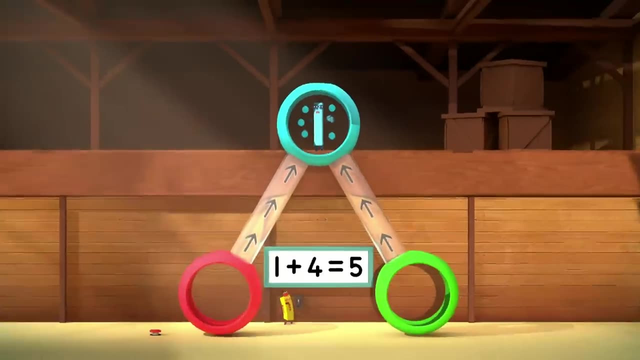 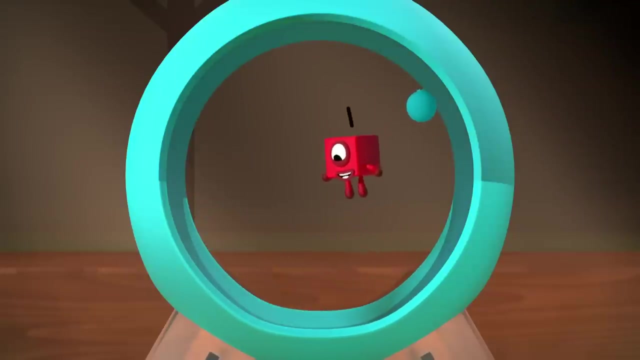 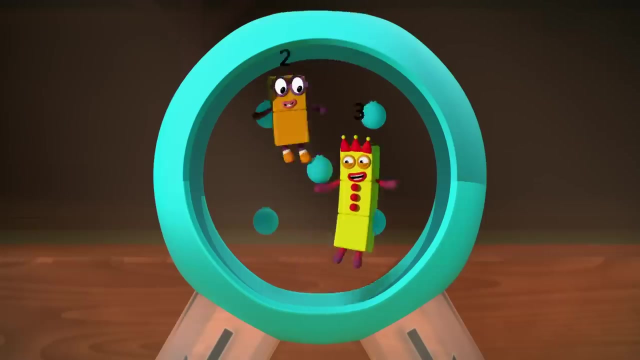 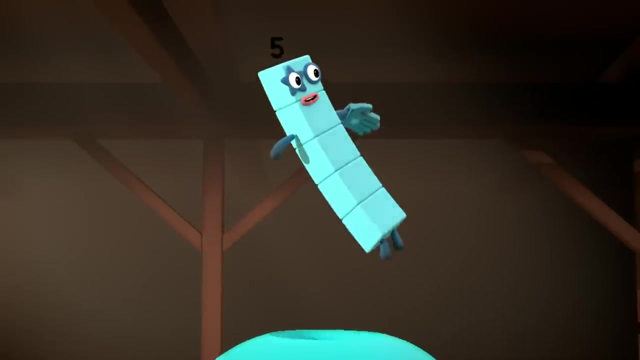 Five equals one plus two. One plus four equals five. Yikes, Five equals four plus one. Four plus one equals five. Five equals two plus three. Two plus three equals five. It's going far too fast. Five equals three plus four. 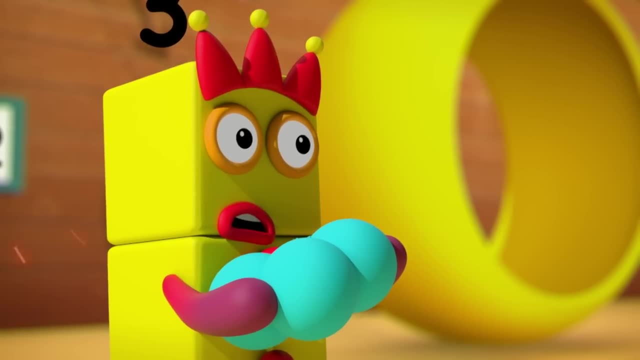 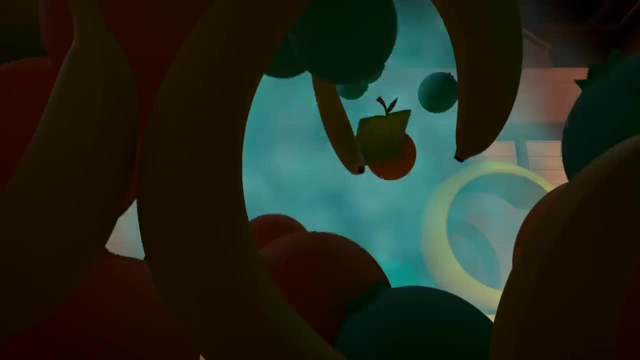 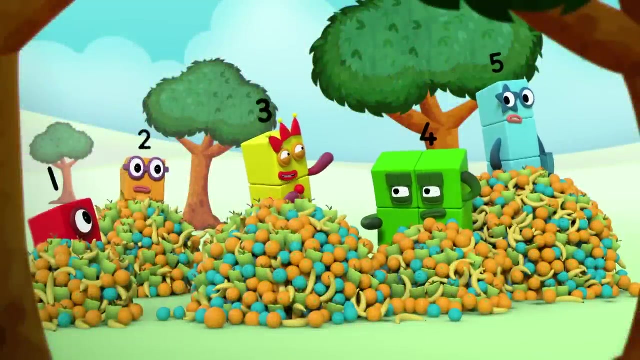 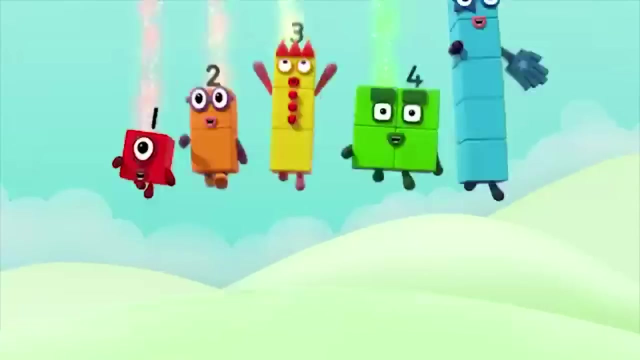 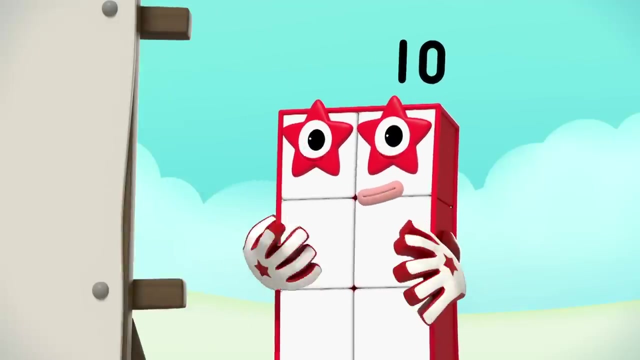 One, two, three, Three. blue bears. Front Front. I told you Easy peasy: lemon squeezy Ow, You can count on us, we're the number box. Oh, I know how to cure hiccups. 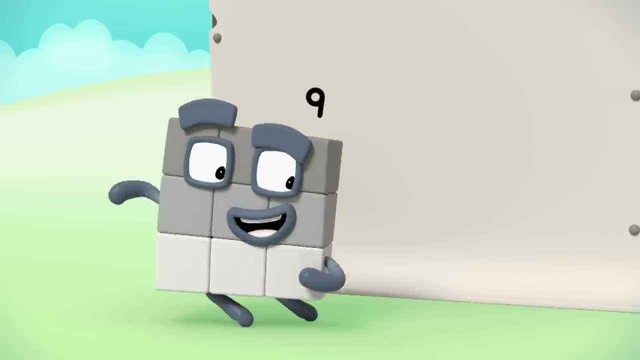 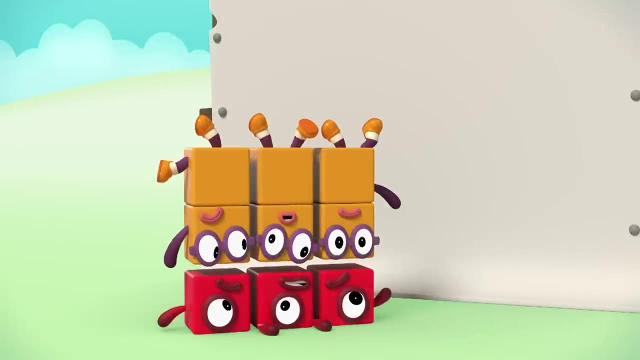 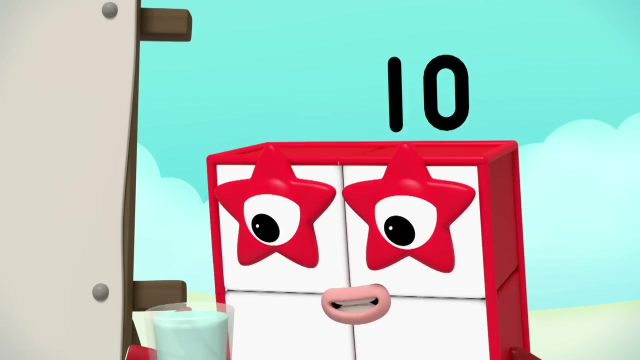 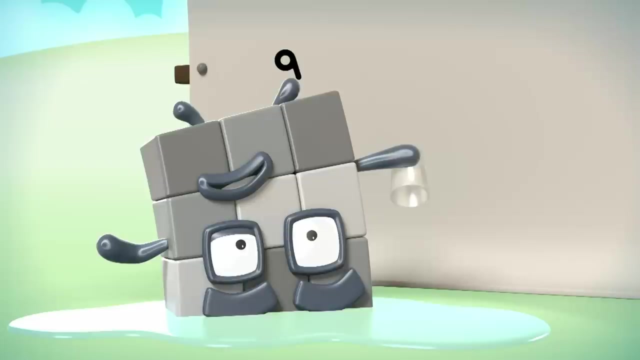 You stand on your head. Huh Huh, I think it's working. Hang on. I know another one. Drink a glass of water backwards Harder than it sounds. Oh Oh, We need help, Have no fear. 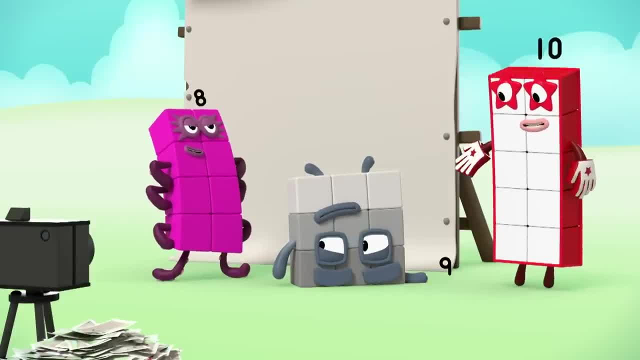 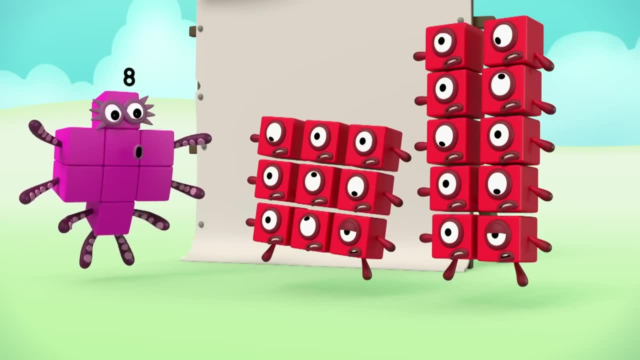 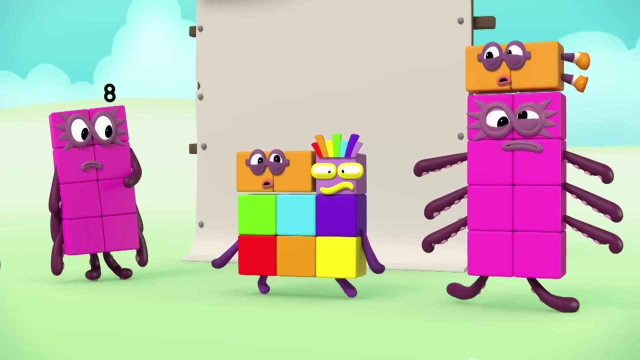 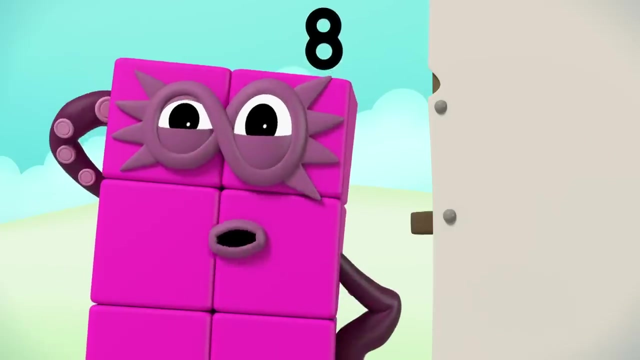 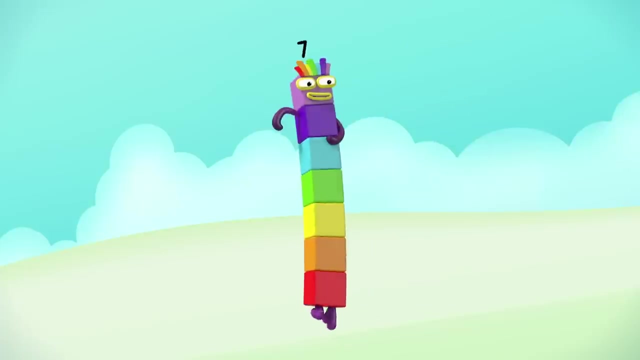 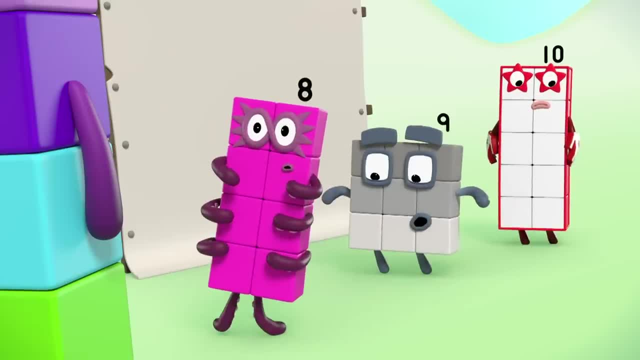 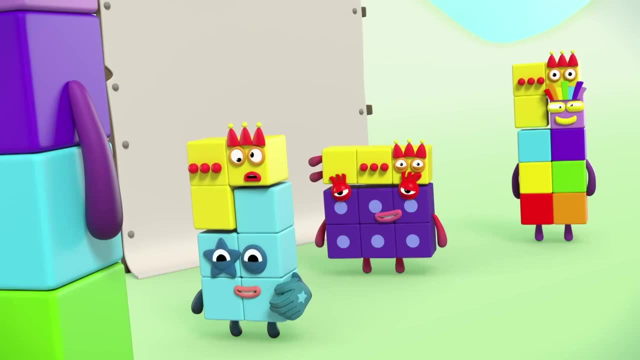 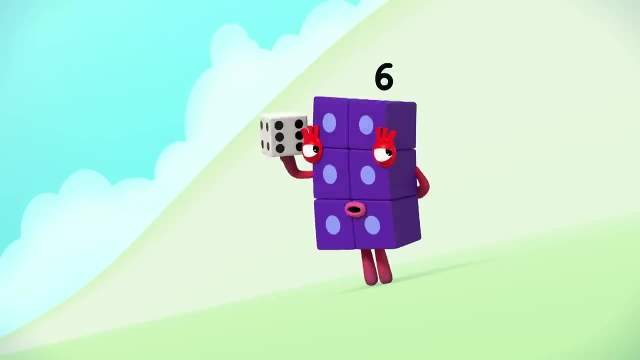 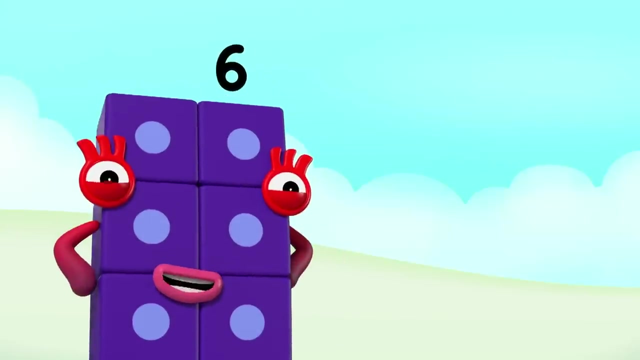 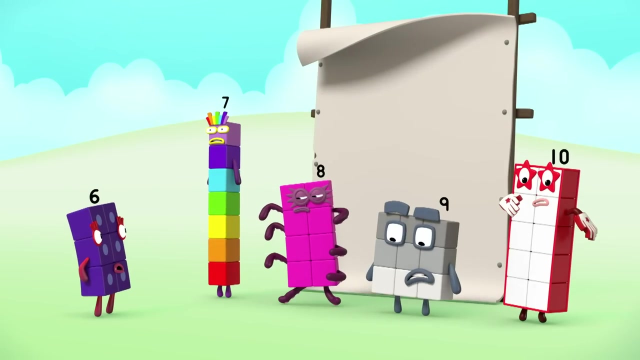 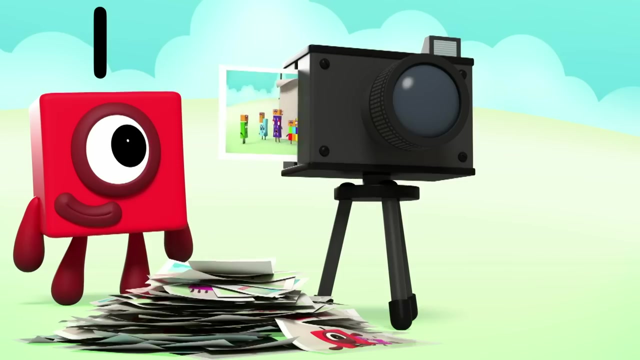 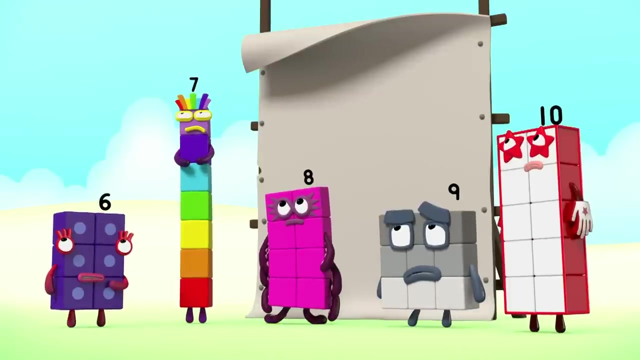 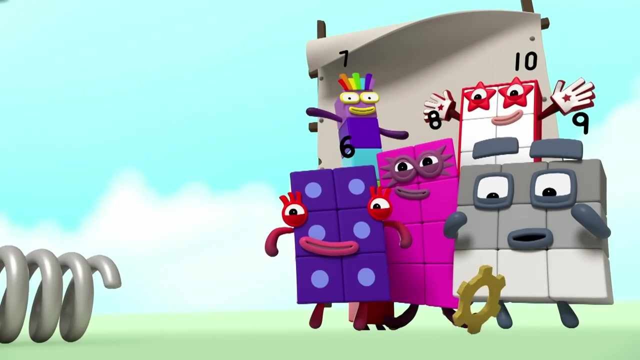 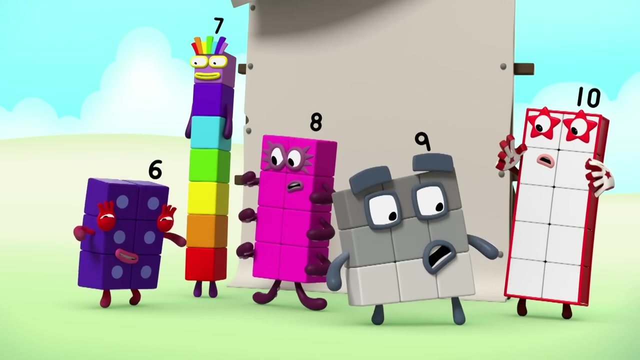 Lucky, lucky, lucky, lucky. look, Oh, Um Oh. I tried that eses Outta my way Coming through. Got six hiccup cures for you. lets roll, Oh Cheese. Great photo, everyone: No more hiccups. 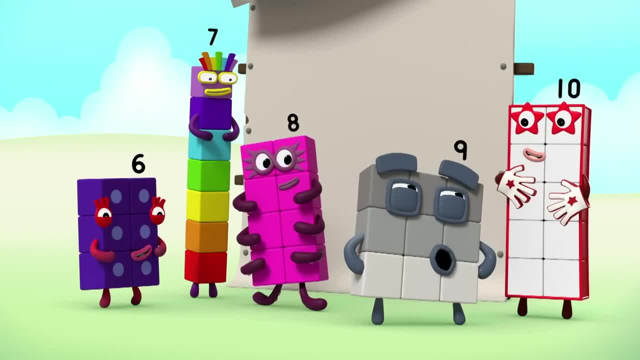 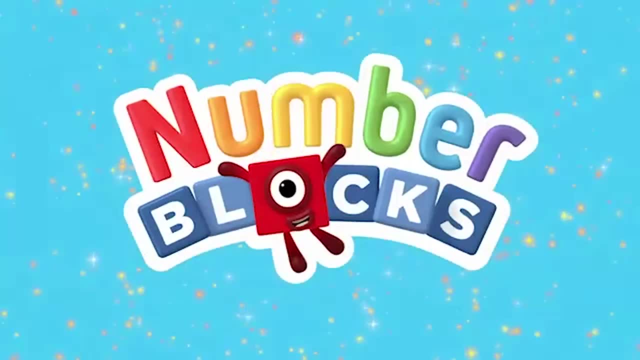 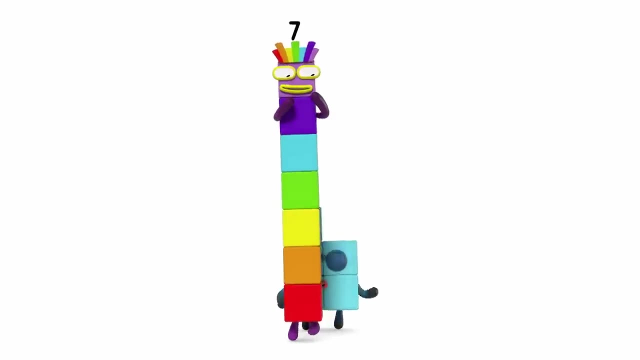 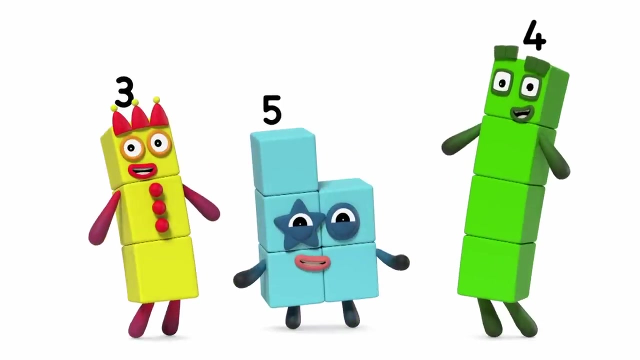 So that's how you cure them. You can count on us. we're the number box. If you're smaller than me, it'll never work, No matter what shape you make. Six won't fit into four's little bed. I can lie down in ten's bed instead. 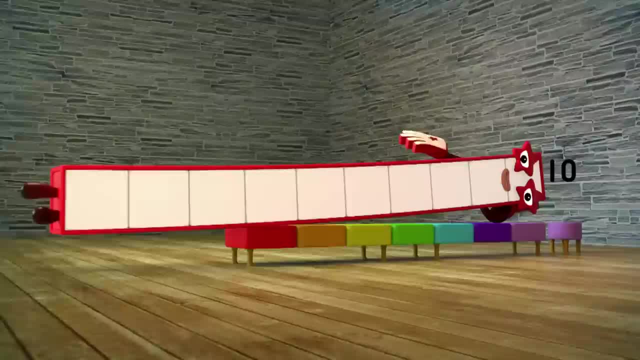 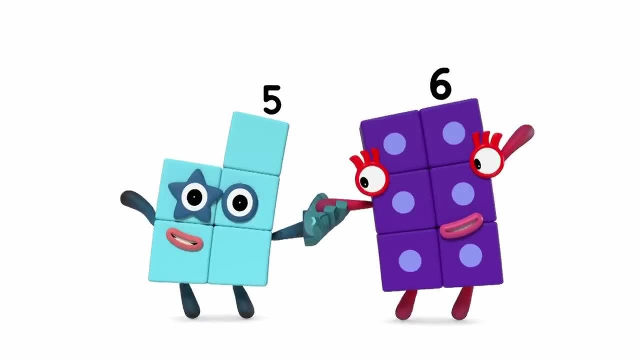 Seven's bed is too small for ten. My feet will stick right at the end. Peek-a-boo, I'm hiding behind you. If you're bigger than me, no one will find you. Where have they gone? Go on, give us a clue. Can you see me? 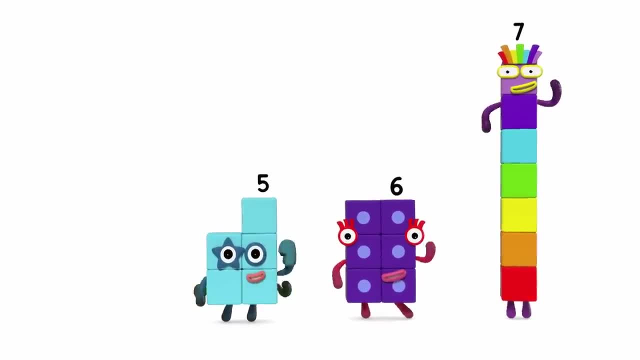 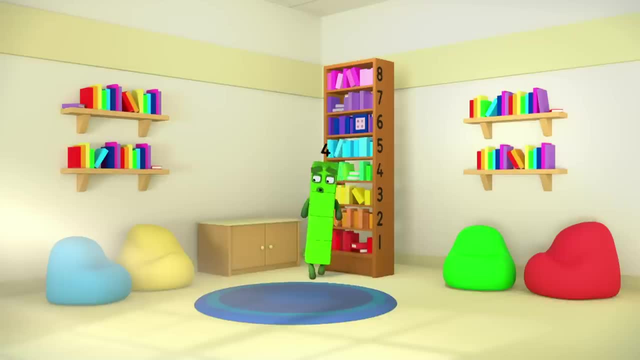 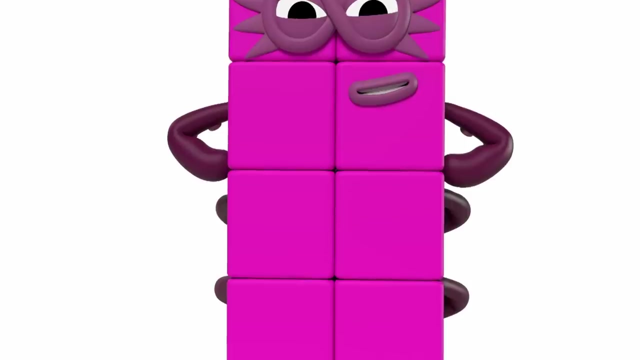 Peek-a-boo, Can you see me, Peek-a-boo? Four can't reach up to six himself. I'll have to leave that book on the shelf. Eight can bend down to reach the book. Six can peek through and take a look, Peek-a-boo, I'm hiding behind you. 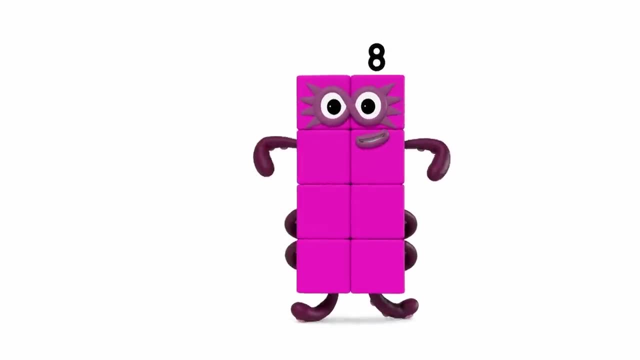 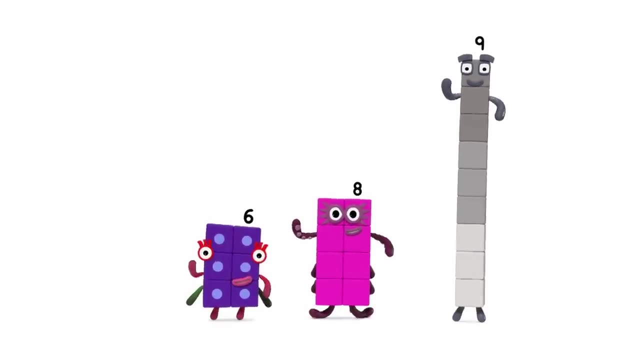 If you're bigger than me, no one can find you. Where have they gone? Go on, give us a clue. Can you see me, Peek-a-boo? Can you see me, Peek-a-boo? Can you see me, Peek-a-boo? 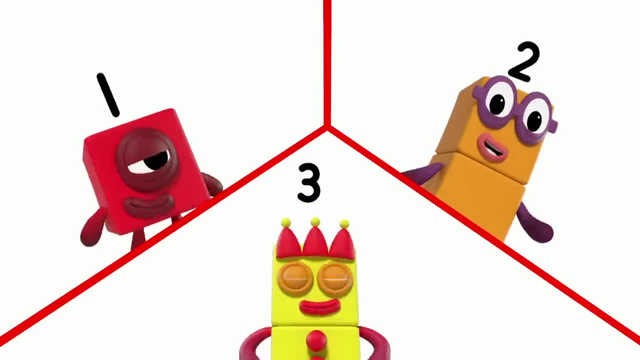 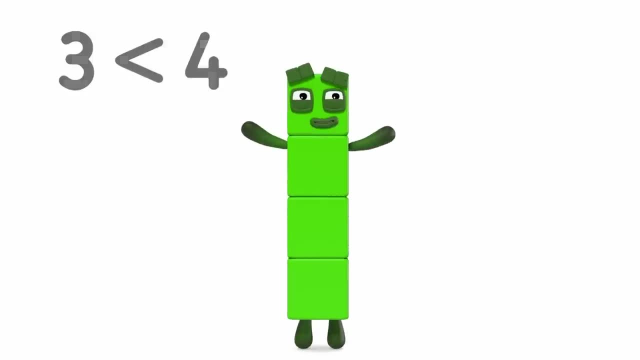 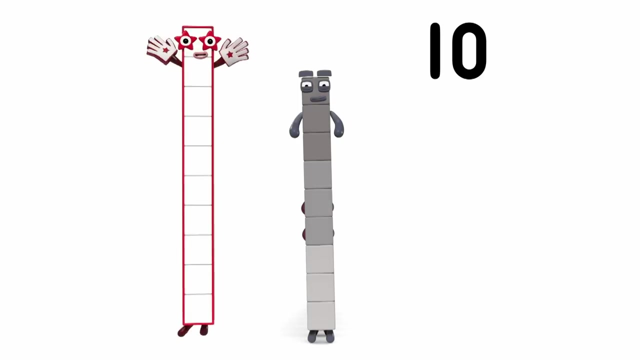 One is smaller than Fewer than Less than One is less than Two is less than Three is less than Four, Five is less than Six is less than Seven And eight is less than Nine is less than Ten, And ten is bigger than More than Greater than Ten is greater than. 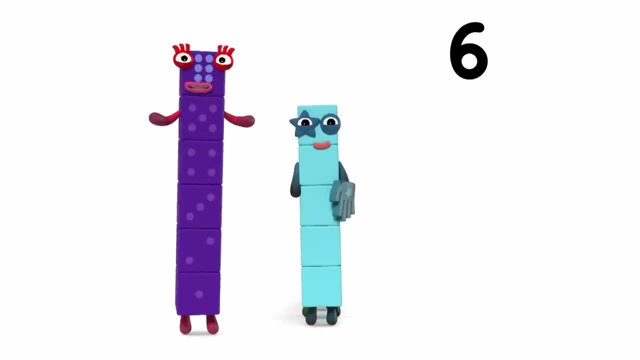 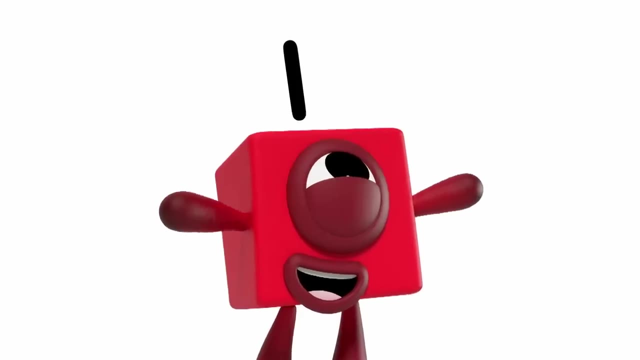 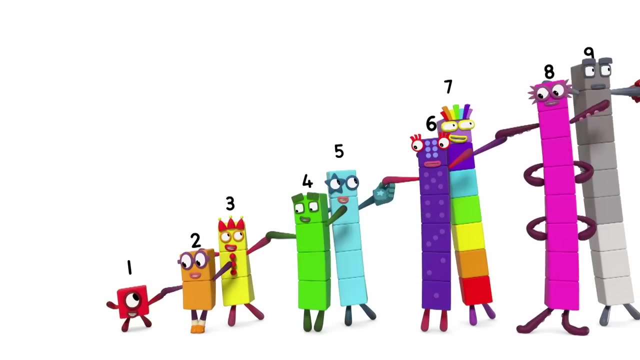 Nine is greater than Eight, is greater than Six, is greater than Five, is greater than Four, is greater than Three And three is greater than Two is greater than One. Peek-a-boo, I'm hiding behind you, Cause I'm bigger than you. no one will find you. 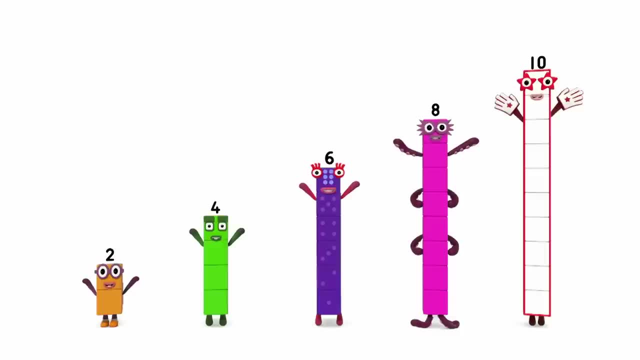 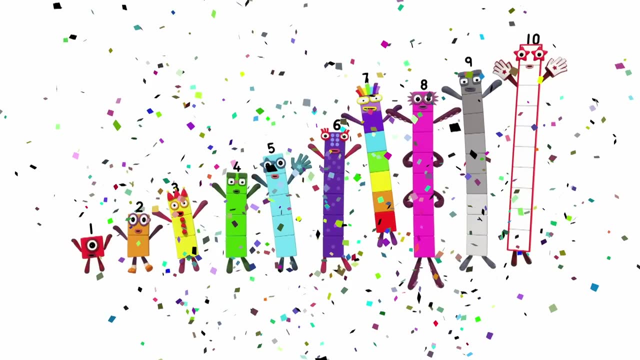 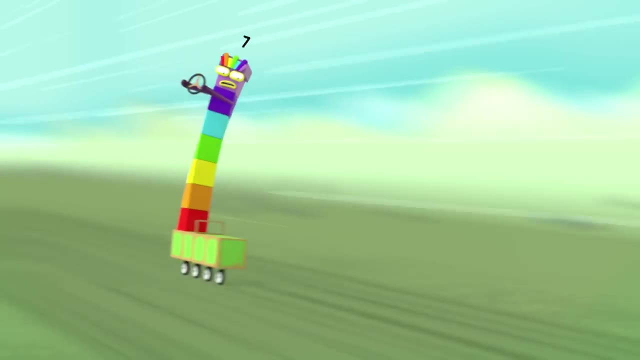 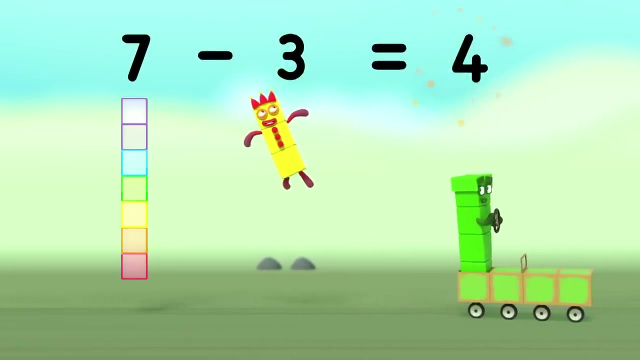 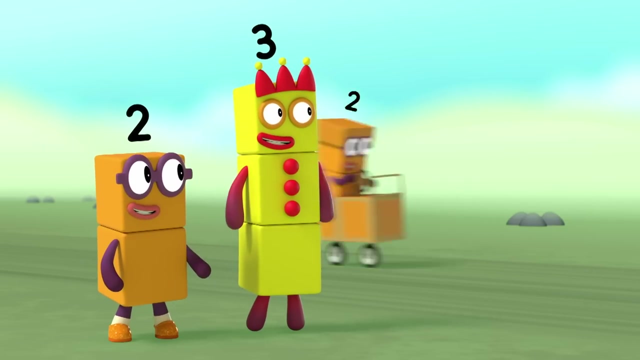 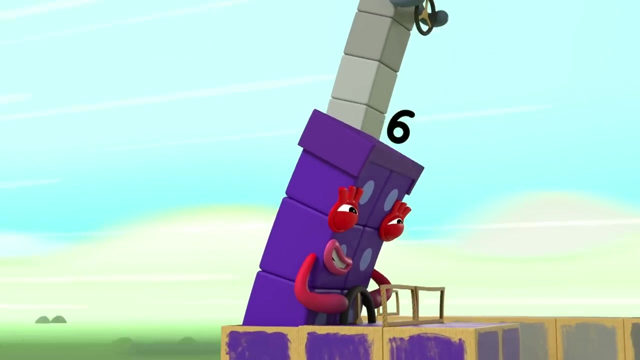 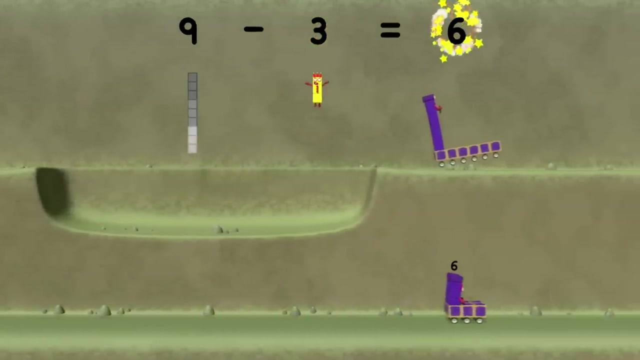 Where have they gone? Go and give us a clue. Can you see me, Peek-a-boo? Can you see me, Peek-a-boo? Count on us. we're the number box: Nine minus three equals six, And the double dips: Six minus three equals three. 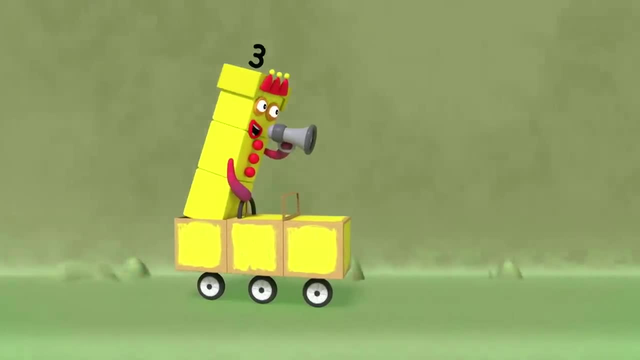 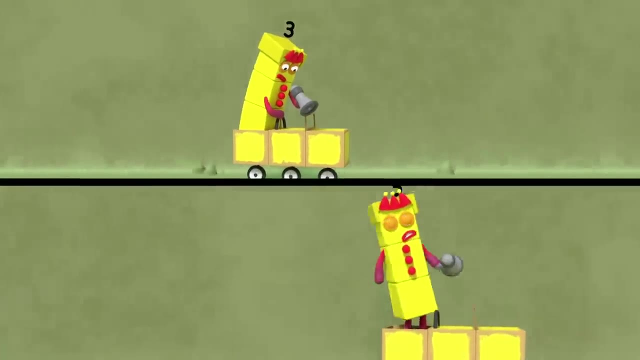 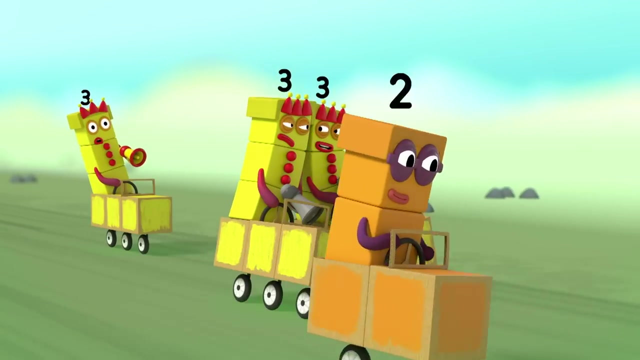 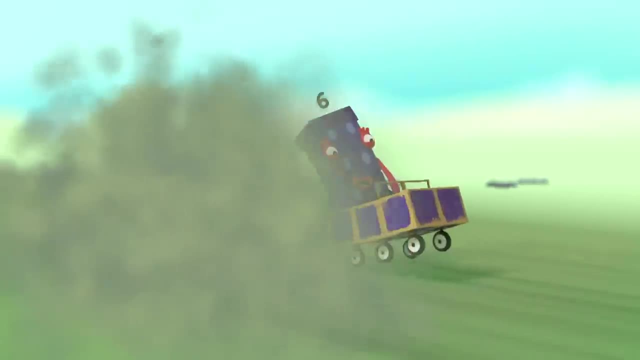 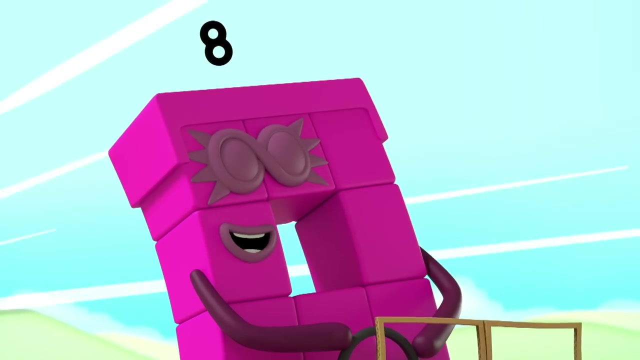 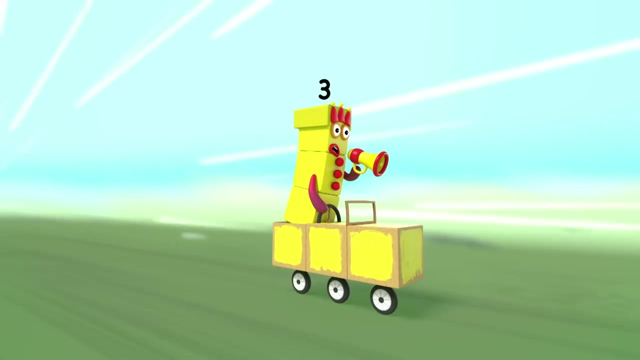 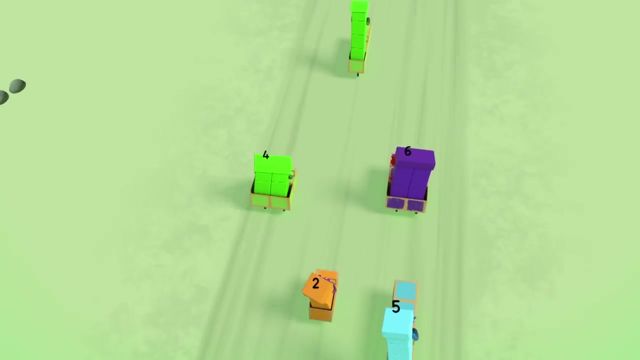 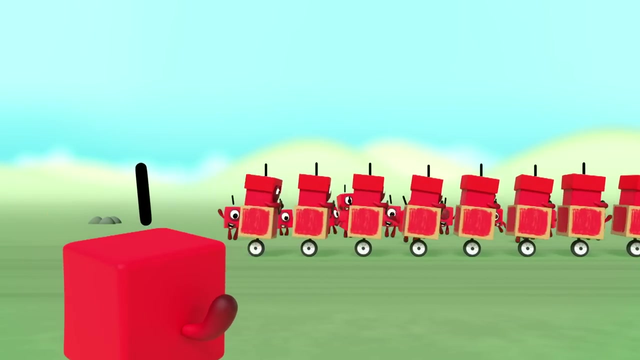 Three equals three equals me Back in action And with the finish line in sight. It's four in the lead. Then I need a breather Octoblock coming through, Uh-oh, And it's one in the lead, Followed by one, But here's one coming up on the inside. 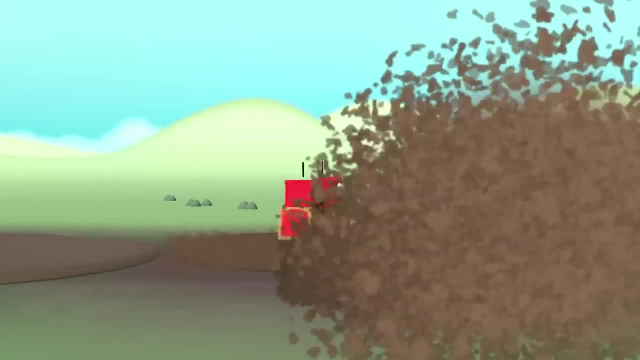 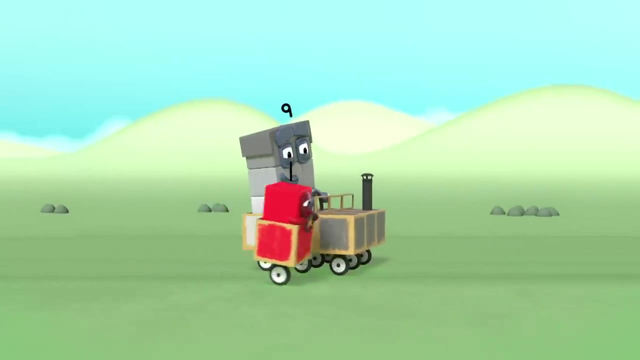 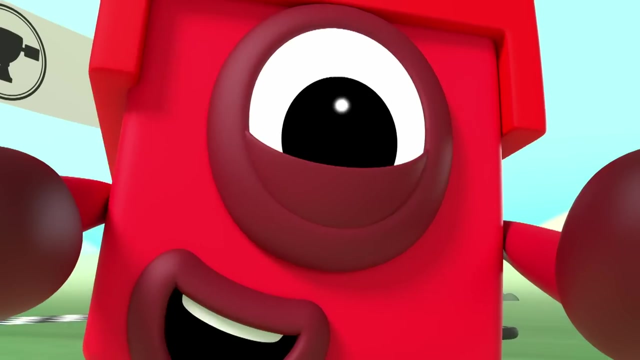 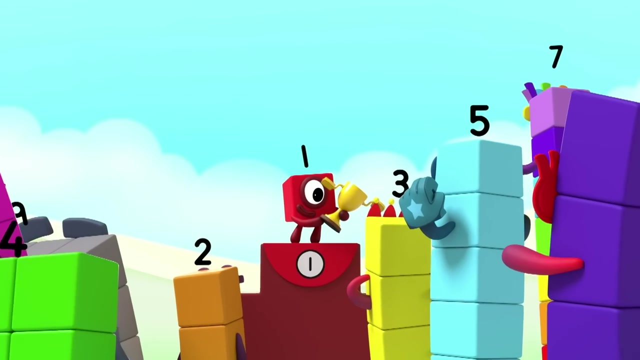 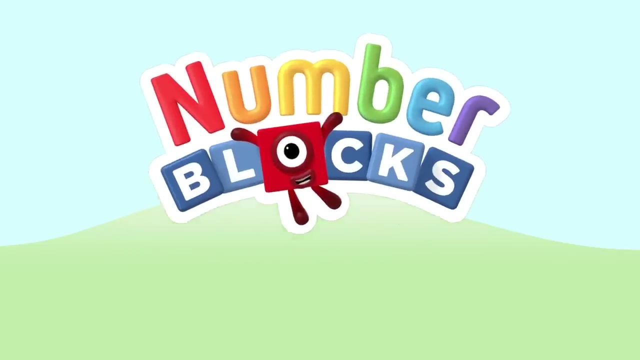 Nine ones equals Nine. Nice day for it, I'm first, I'm first, Oh yeah. Well, I said only one can lift the trophy, And I was right. Oh Right, you've done well. Oh, One, two, three, four, five. Number blocks. 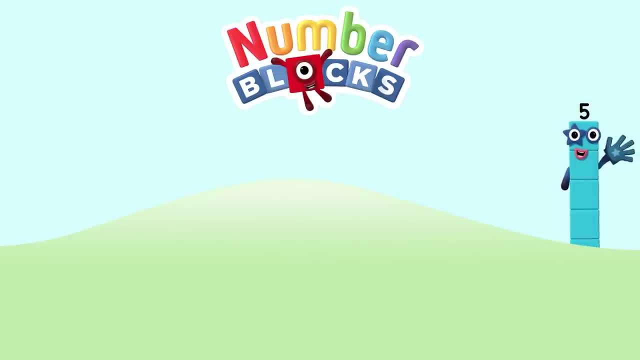 One, two, three, four, five. Number blocks: One and another. one is two And another one is Me. That's three, Five, four, three, two, one. You can count on us, we're the Not-A-Vox.